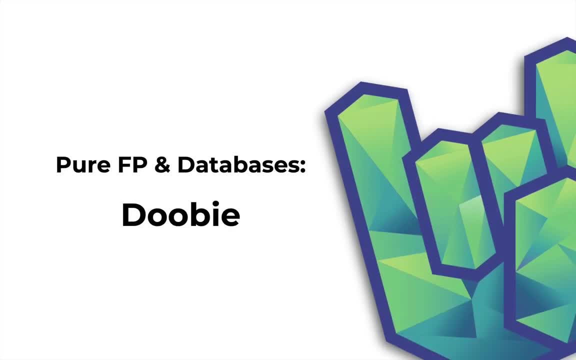 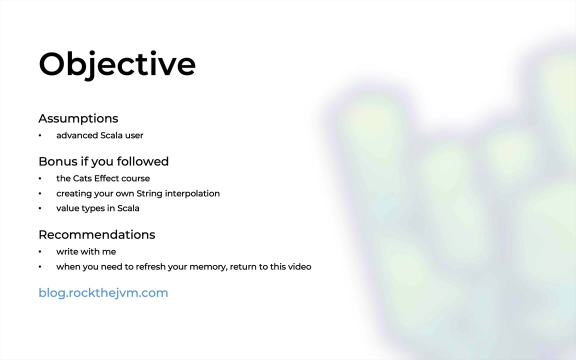 Hello, ladies and gents, this is Daniel for Rock the JVM, and in this video we are going to do pure functional programming with databases in Scala with a phenomenal library known as Doobie. Now, this tutorial is probably going to be a little long and it's for the advanced Scala user, So 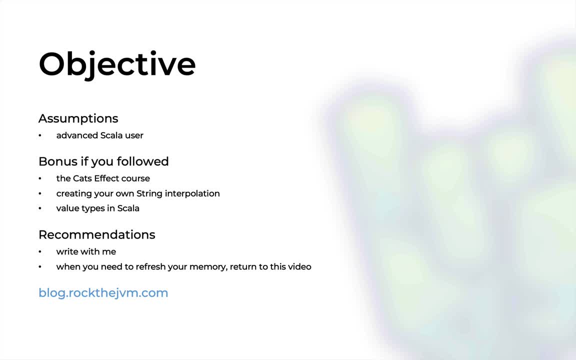 this video, or set of videos, depending on how long this is going to take- is for those of you who are very comfortable using Scala- And we're going to use quite a lot of concepts that I've talked about in other places, especially if you follow the Cat's Effect course- this will be the most 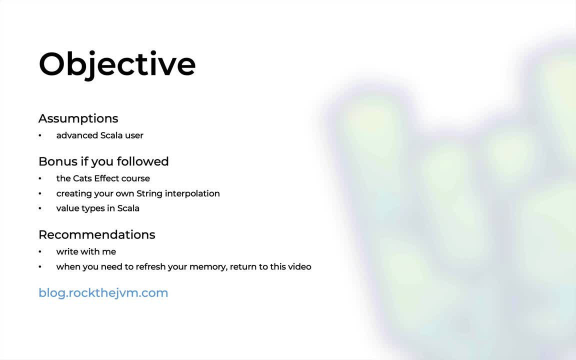 appropriate for you. We also talked about how to create your own string interpolation and value types in Scala, among other things on the YouTube channel. As always, I recommend that you write code with me in this tutorial, because we're going to write quite a bit of code And whenever you need. 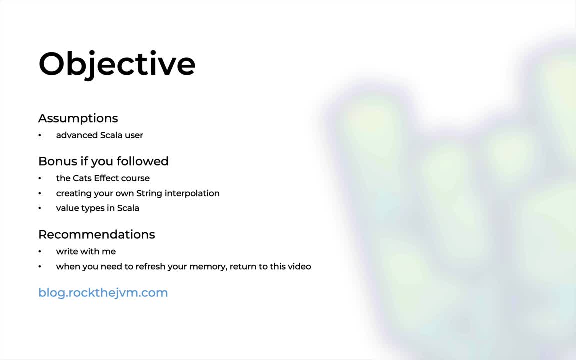 to refresh your memory or need a teammate to learn Doobie. just refer back to this video or to the written form at the blog, with the link in the description And, if you have any questions, the link in the description which, by the way, I recommend that you have handy because we're going. 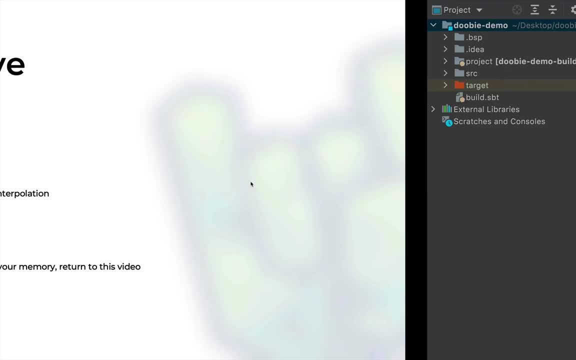 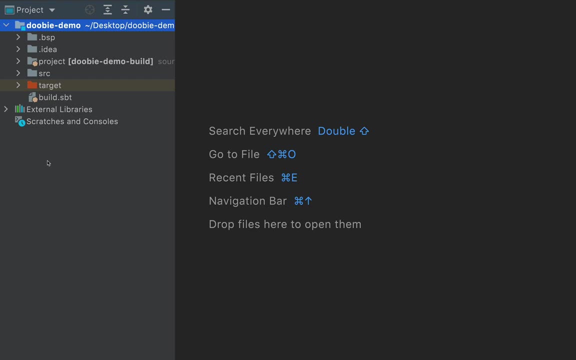 to copy some configuration code. All right, cool. Now, without further ado, I've created a new project for this particular tutorial. So this is an empty Scala project And I'm using Scala 2 for this tutorial, although I'm pretty sure the same code could work on Scala 3.. I haven't tested this. 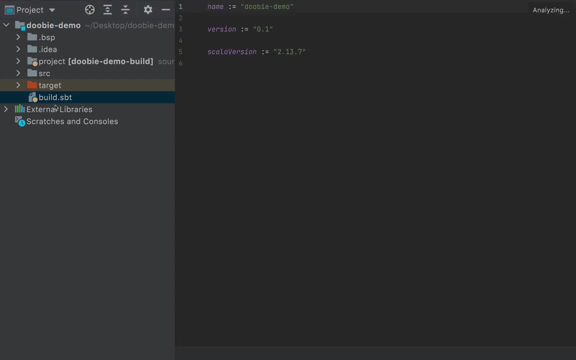 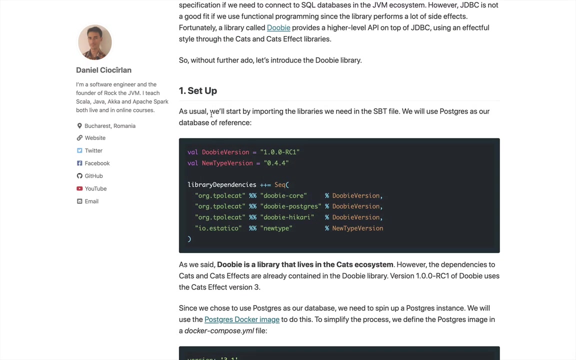 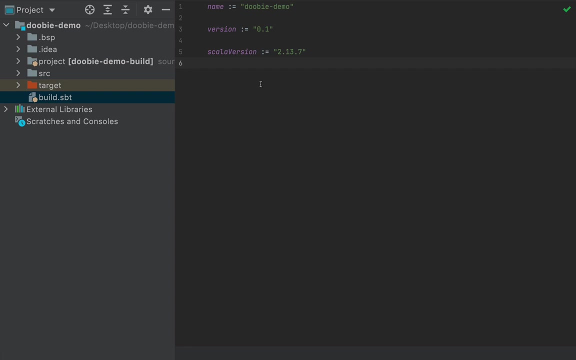 because my dev environment is acting up And the first thing that I'm going to do is add the library definitions under my buildsbt, which you can find in the written version of this tutorial. So here, at the very first code box, you can simply copy that and paste the contents at the end of 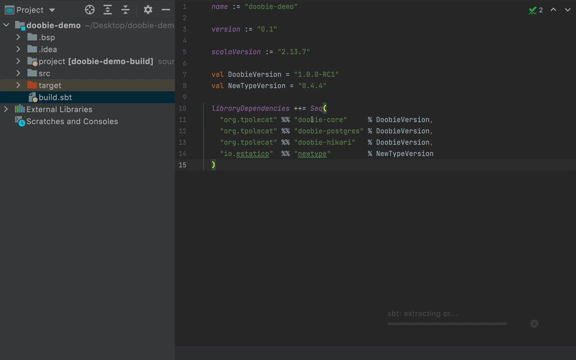 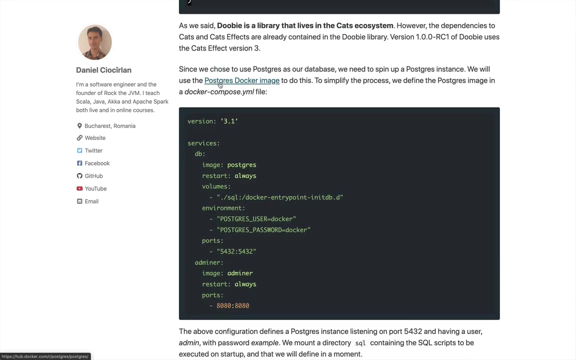 your buildsbt. hit this little refresh icon And in just a few moments we're going to have all the libraries downloaded automatically. Cool, While the SBT is downloading all the library definitions, we're also going to create a Docker container so that we can have a database to work with. So I'm going to copy this content over: 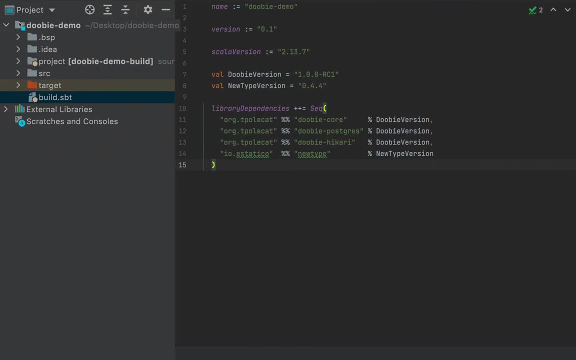 here, which is a Docker Compose- YML file, And under the doobie demo, or at the root of my little project, I'm going to create a new directory. I'm going to call this Docker, And under Docker I'm going to create a special file whose name is docker-composeyml. Pretty sure you're familiar. 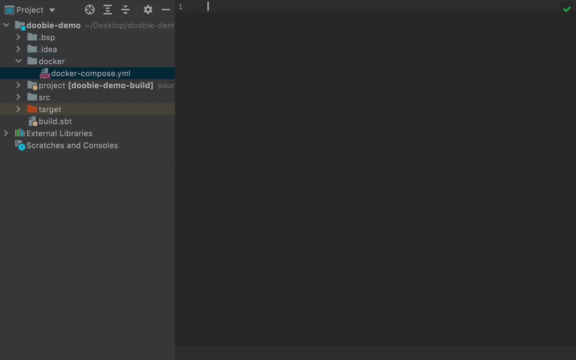 with this kind of file. The name is important And I'm going to paste the contents here. So the Docker Compose YML specifies that the image is Postgres, which Docker can automatically find The volumes means that we have a folder or a directory that we're going to mount inside the Docker container we're going to create. 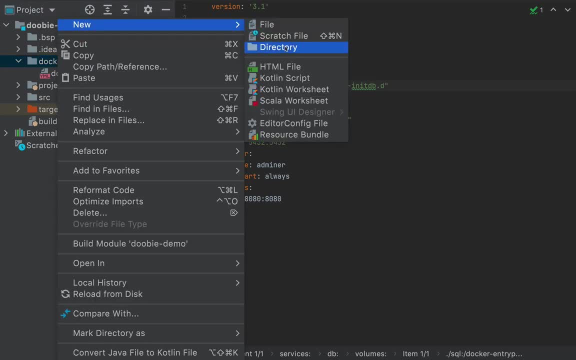 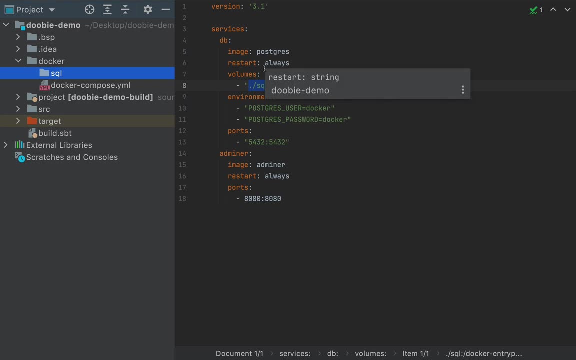 a SQL directory under Docker. So I'm going to create a new directory here. I'm going to call this xml database And let's see what that looks like, And it will store the files that are in the file that I'm going to be working on, our Docker container. So I'm going to say xml target for. 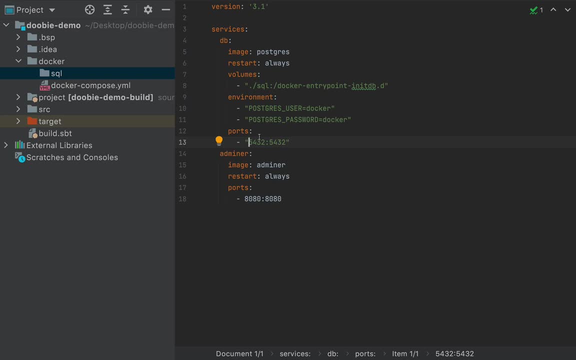 docker-compose-yml. I'm going to say xml target for docker-compose-yml and then put the own address here And I'm going to put my name here, I'm going to put my password here and I'm going to say my-imdbsql for this database And then I'm going to put an address here under my existing. 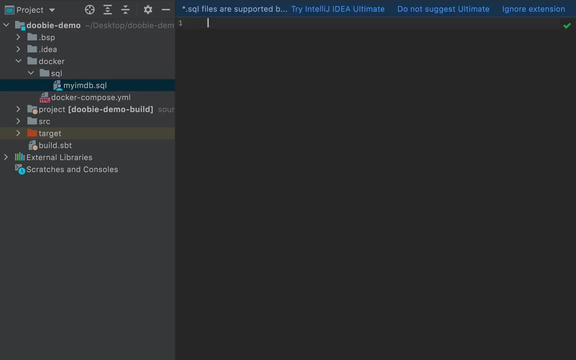 whoop there, And then I'm going to put a new current folder and then I'm going to put my name into that folder And then I'm going to put my current я thứ tres command. I'm going to put my name into the. 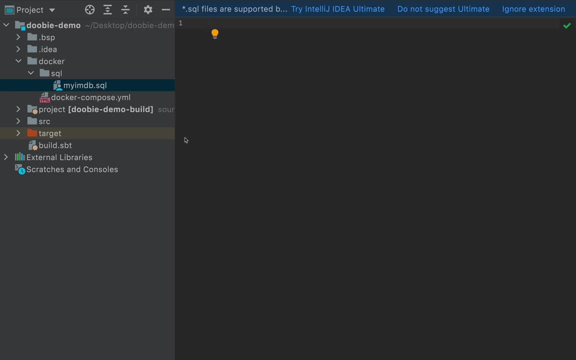 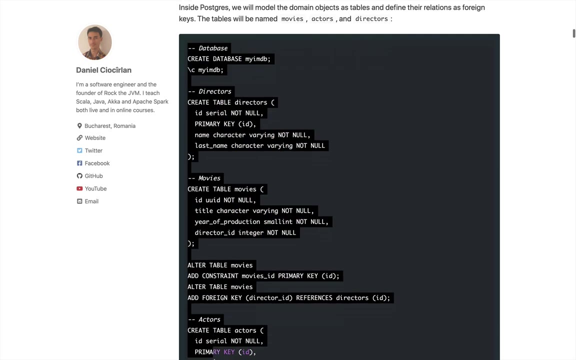 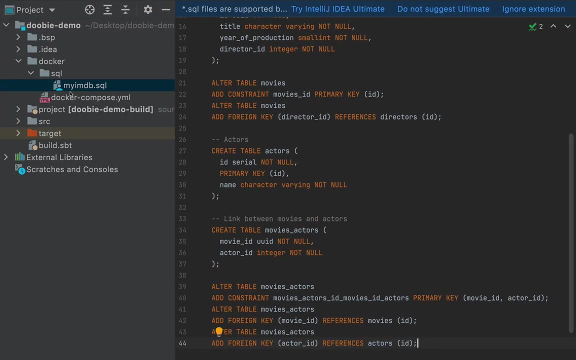 actors, movies, directors and that sort of stuff for a fictitious imdb kind of application that we are going to create. and right underneath that we have a big code block that i'm going to copy and i'm going to paste that inside my imdbsql. so this is the database definition, which has: 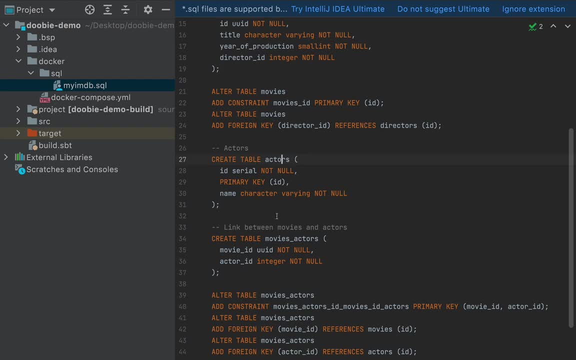 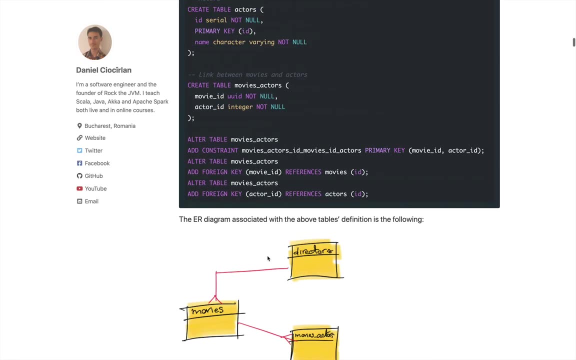 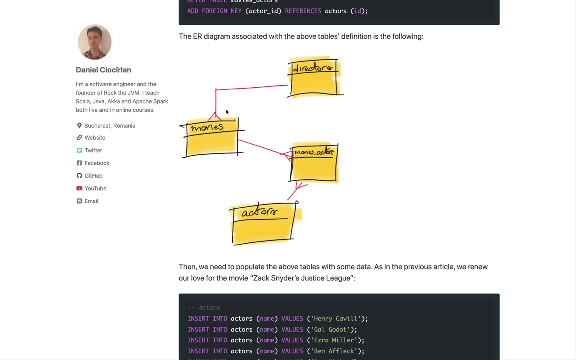 some tables- directors, movies and actors, and movies, actors- and we also have foreign keys between these tables so that we can query them easily. the diagram looks like this: where we have directors and movies, so every movie has one director. a director can direct multiple movies and movies and actors are in many to many relationships, which is why we have this. 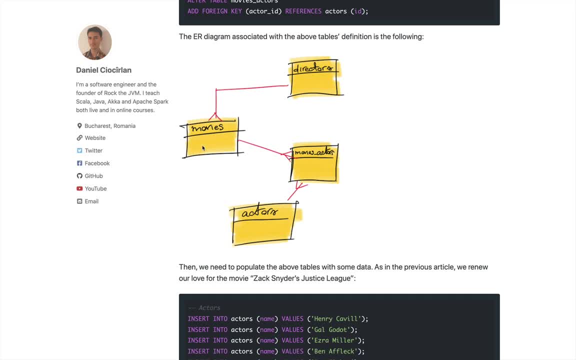 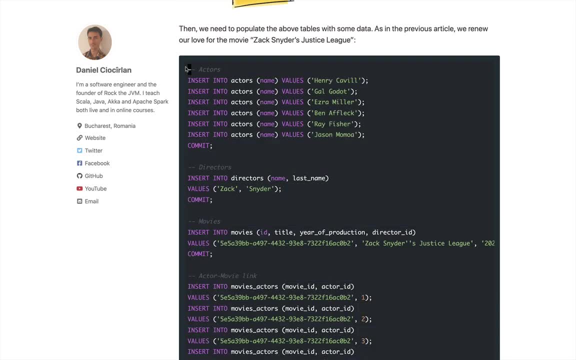 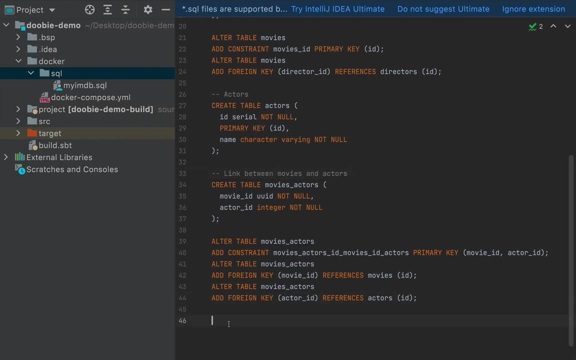 intermediate table: movies underscore actors to simplify those relationships. and now i'm going to add the actual data that will sit inside this database. so i'm going to copy this whole block of code and then i'm going to add that at the bottom of my imdbsql. so this 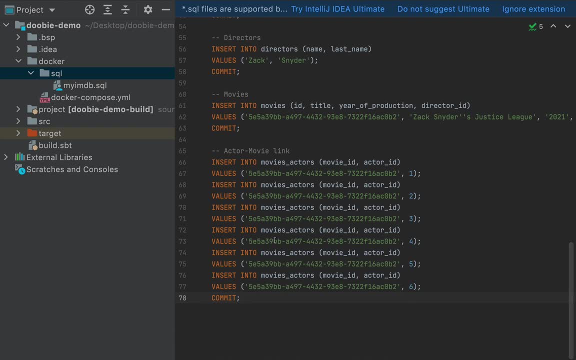 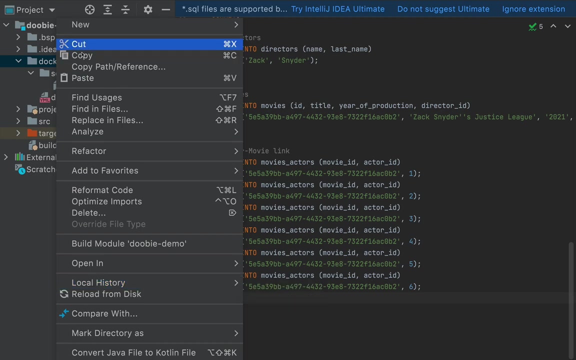 is going to be the sql script that is going to be executed when the posgres database container is going to start up. cool, now i'm going to navigate to this docker folder here, the docker directory. so i'm going to say copy path and i'm going to copy the absolute path and in a turn, 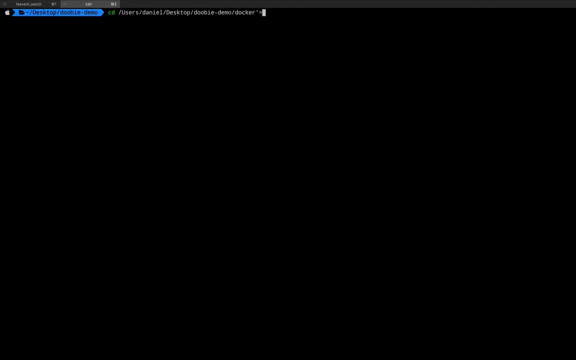 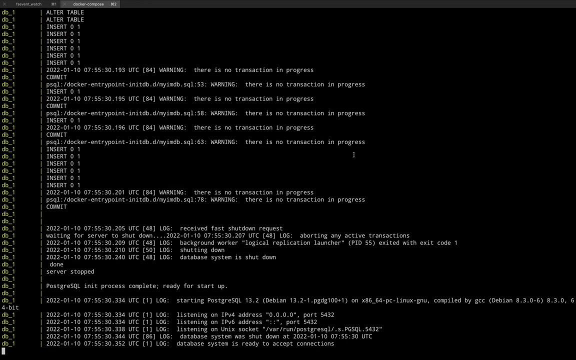 and in a terminal i'm going to navigate here to the docker directory and then i'm going to say: docker, dash, compose up so that docker can fetch the appropriate image and start the posgres container. yes, i will allow docker to access everything, and if you see this sort of output, 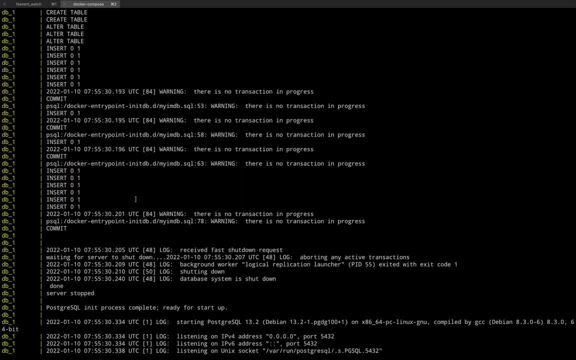 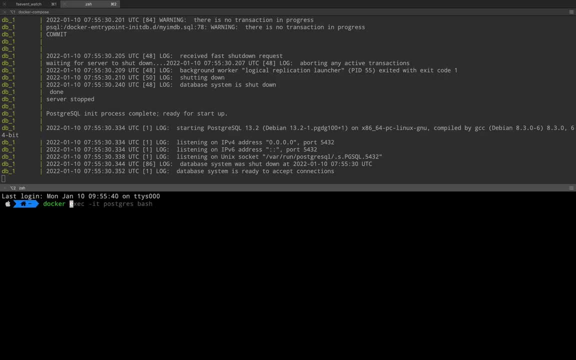 where we see alter, table and commit, then that means the docker database was correctly created. and i'm going to say docker ps to see what kind of docker containers we have. so we have docker underscore db, underscore one- this is the name of the database container- and i'm going to say: 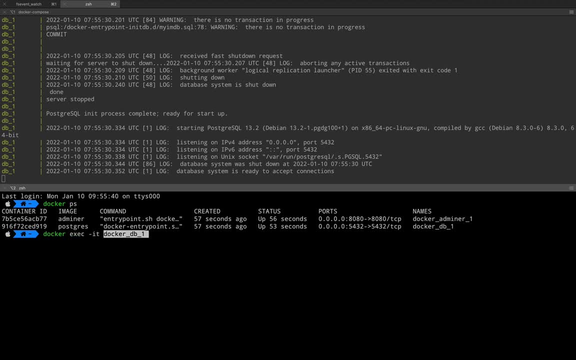 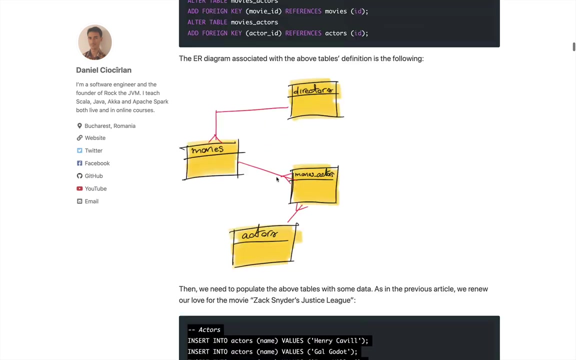 docker exec, dash it this thing, and then a bash, and now i have root access inside the docker container and i'm going to say: psql: dash u big u, docker, dash d the database, my imdb. this is the name of the database that we created at the beginning of 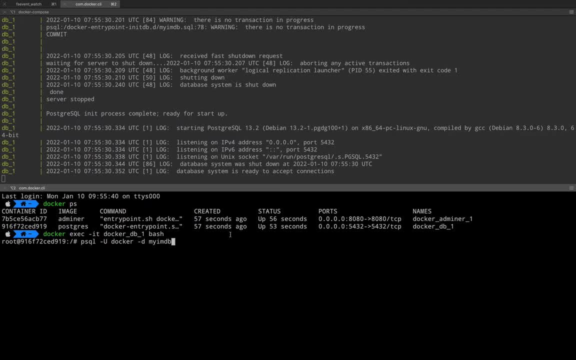 the sql script, the create database, my imdb, so i'm going to connect to this database so that i can query something. so if i do select star from actors, we have a bunch of actors already created for us by the script that i added at the beginning. all 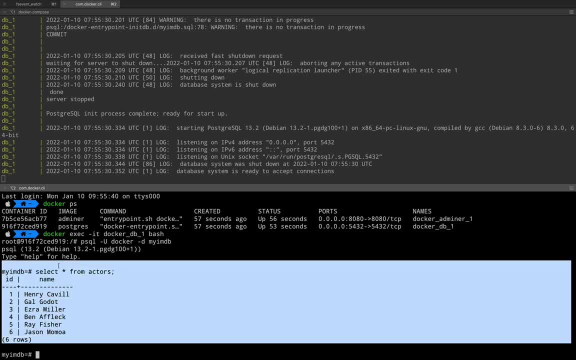 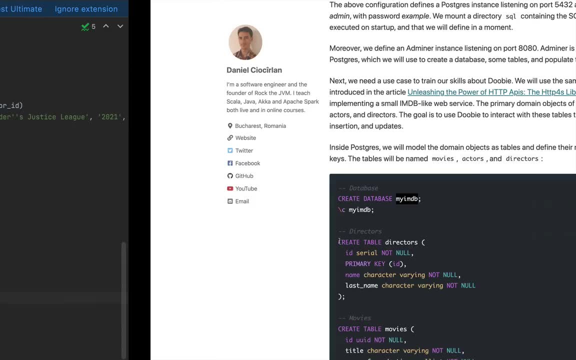 right. so if you run all these commands and you see this kind of output, then that means your database successfully created, and this is a prerequisite for what we are going to do from the code, that is, from the scala code. all right, so the docker container is running and under source main scala. 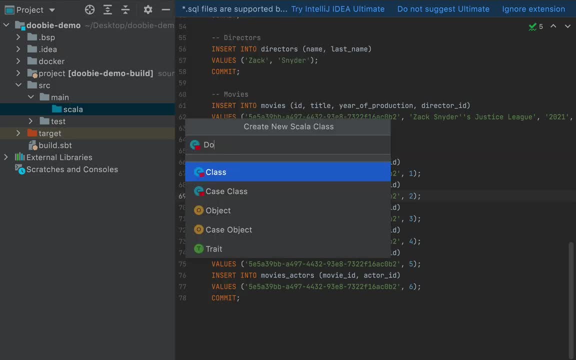 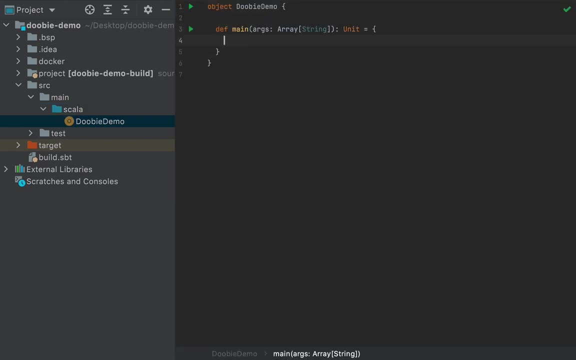 we are going to run a new skull application. i'm going to call this doobie demo, make it an object, and i'm going to create a main method in case we need to test some stuff. now. the doobie demo will actually be an i o application, because doobie 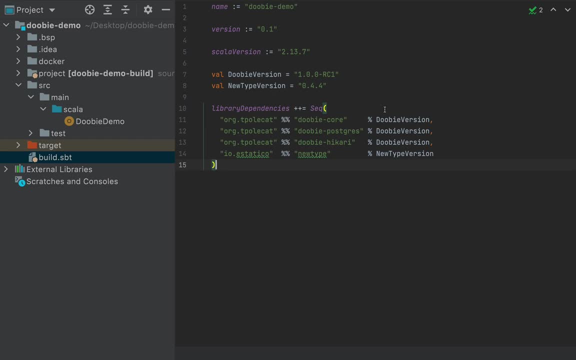 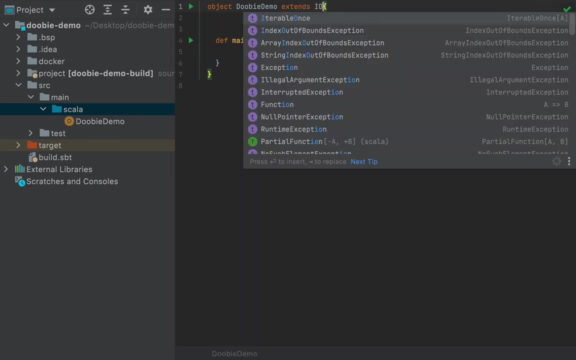 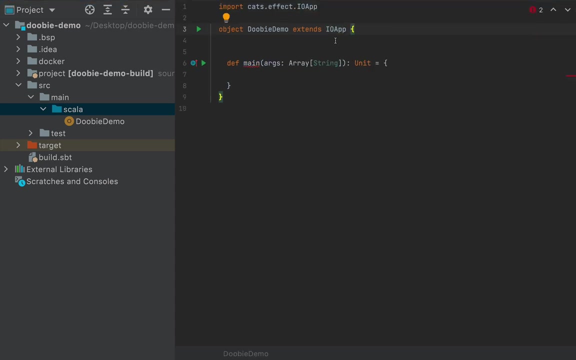 as a library is based on cat's effect. so if we want to run a cat's effect application, i'm actually going to say object doobie, demo extends and i'm going to have io app that you can find from cat's effect and cat's effect being a dependency, it's already added for us inside the dependencies of. 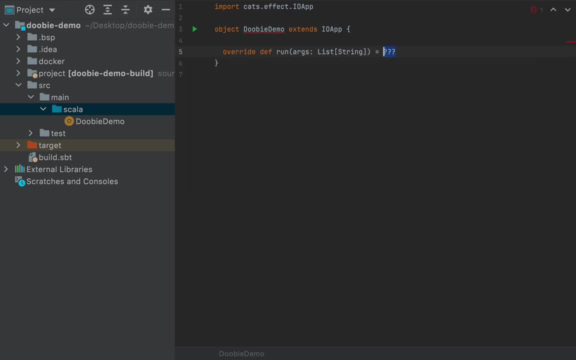 our project and io app has a method called run which returns a special data type called an io. so this is an io of exit code and io is very important. it's the fundamental data type of cat's effect, so we will naturally import that and we are going to say, for instance: uh, io with println. 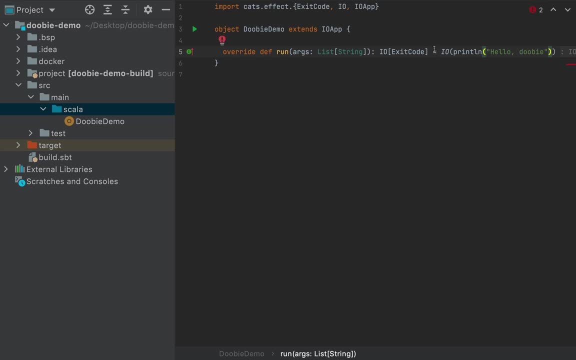 hello doobie. and then i'm going to turn this io, which is an io unit, as exit code dot success. so this will be a valid io application in cat's effect and we're going to test that to make sure the application has all the appropriate libraries correctly downloaded and installed. it takes a little while. 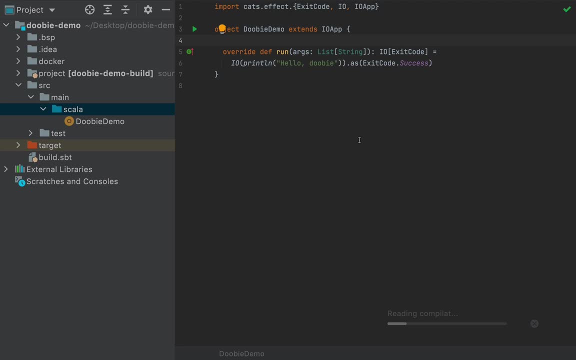 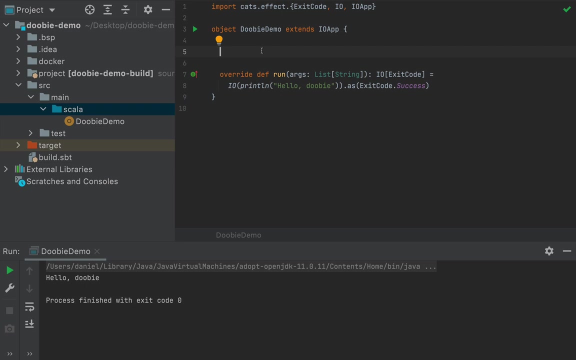 for the compiler to warm up, and after that the compilation will be a little faster. all right, so we have this little string and finally, after eight or so minutes of just setting things up, we can write some actual code. now, how do we interact with a database using doobie? well, we are going to need 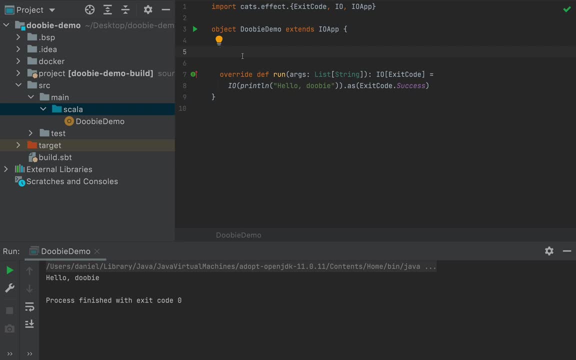 what is called a transaction. so we're going to use doobie as a database and we're going to need a data type called a transactor. a transactor is a data type that will allow us to run a connection to our database, run a query and return some values based on that connection. so i'm going to call this. 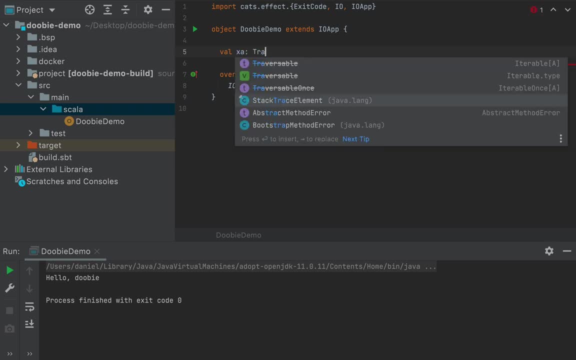 transactor, xa, and the type of that is transactor. and transactor takes a higher kind of type which we are going to use as the type of cat's effect, which is io. and for those of you familiar with cat's effect, you know what io is. 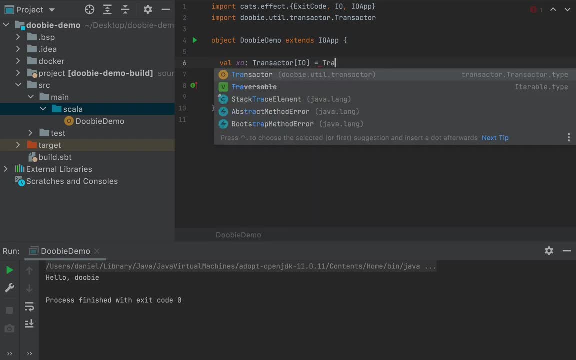 and we're going to run the following: i'm going to say transactor, i'm going to say from driver manager, and this will take as effect type io and as arguments we are going to pass the driver class name, so the driver is going to be orcposgresqldriver. 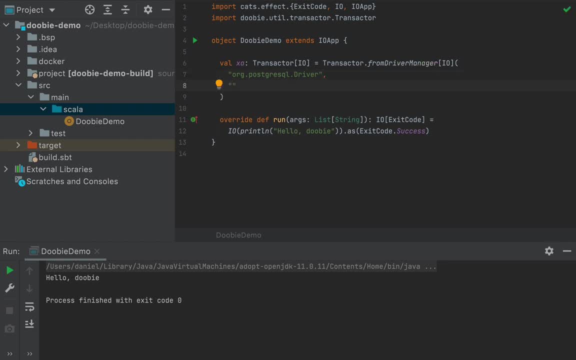 we're going to need the url for the, so this is JDBC, colon, postgresql, and then the URL of the actual database. so this is going to be slash, slash localhost, 5, 4, 3, 2, slash my imdb, or you can simply say my imdb. this is going to fetch the localhost and the username. 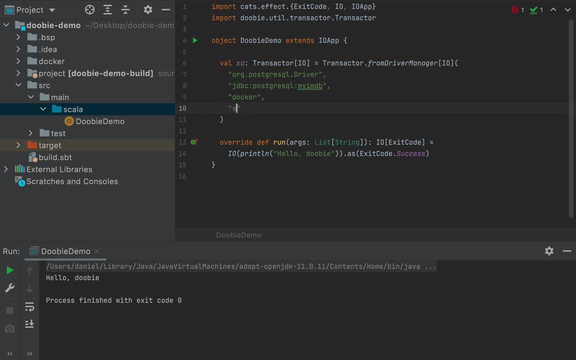 which is docker, and the password, which is again docker. so this is a transactor. now, this is an effectful thing, because when you run an actual query you're going to return an effect. so this will not actually run that particular query until you evaluate that effect, which of course can produce side. 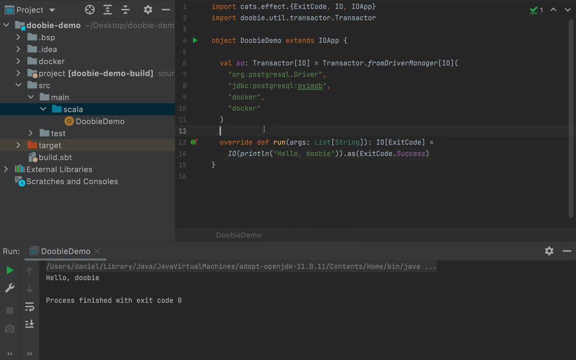 effects, cool. now if you want to run an actual query on top of the database, you will need to use this transactor. so I'm going to define a method. let's say, find all actor names. this is going to be an IO of whatever kind of value you want to return after that query. 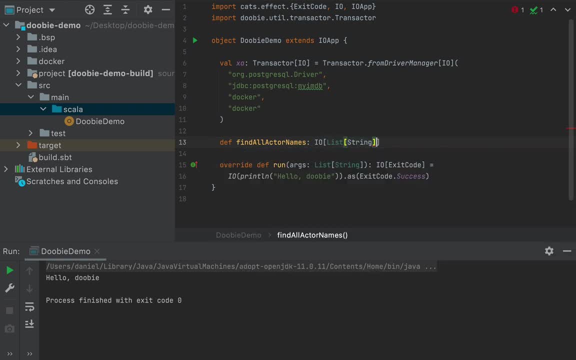 let's say we want a list of strings and I'm going to define my actual query. so I'm going to say: let's call this query as SQL quote and notice that we are now using a custom interpolator. all right, and in order to do that, we are going to 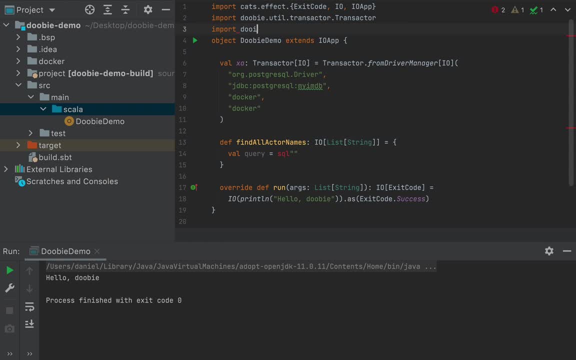 run a bunch of imports. I'm going to say import doobie dot implicits. so doobie implicits everything which will unlock the custom sequel interpolator as being an implicit class over the string context. you probably saw the custom string interpolator video on the rock, the JVM channel. if not, I recommend you. 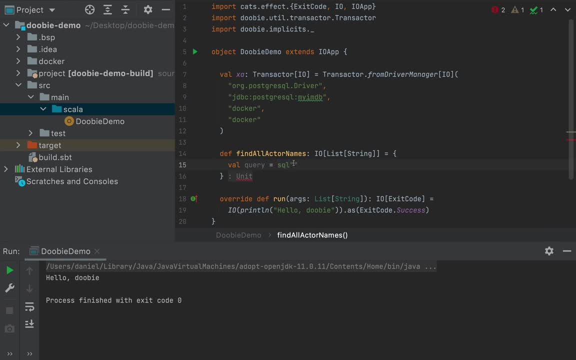 do that if you haven't done that yet. it's pretty cool that you can create your own custom interpolators on top of what Scala naturally offers. so, in any event, I'm going to run my sequel query as select name from actors. this is the actual query that I would write in an 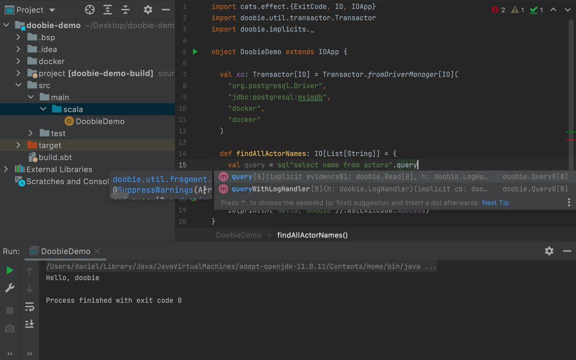 actual database and then I'm going to say dot- query of type string. so I'm going to write the type parameter here and I need to return an actual list of strings by saying: let's call this action as query dot to list. so this will be a very interesting type called connection IO. 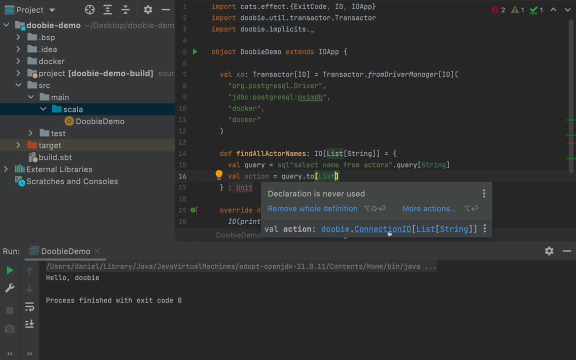 with list string. so this will be an effect full thing which will return a connection that, if run, will return a list of string as a result. so then, as the effect that I want to return at the very end of this method I'm going to say, I'm going to say actiontransact and I'm going to pass this transactor as argument and the end. 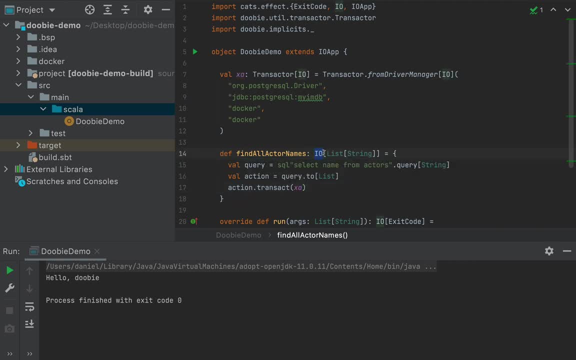 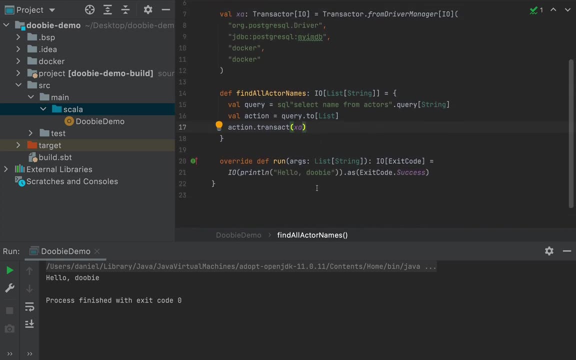 result is that I'm going to return an effect which, when evaluated, will return a list of string after running this query on top of that particular database. So that was quite a mouthful. I'm going to demo that in the code. So in my main method, which is run, I'm going to say find all actor. 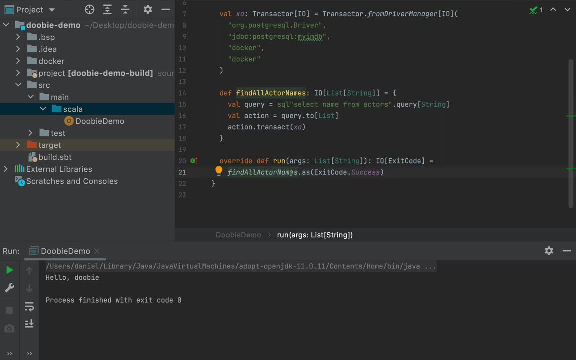 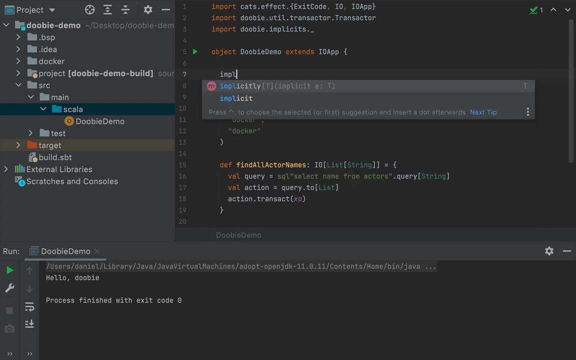 names, which is an IO list string. Now I would like to print everything that I find from the database because, as exit code, success will simply not print anything to the console, and I would like to do that and to that end, I'm going to run an implicit class, I'm going to call: 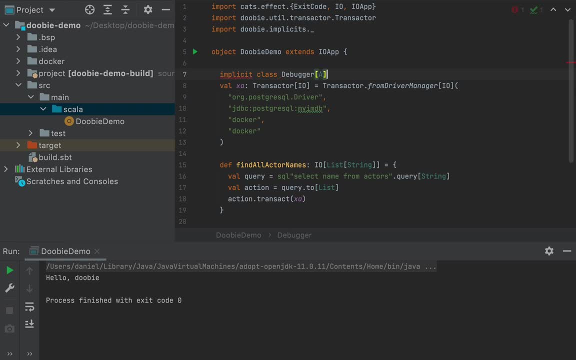 this debugger that takes a type argument a and wraps an IO as an IO a, Just to decorate IOs with an extension method, Then I'm going to call it debug and this will return an IO a and I'm going to run the following and I'm going to say IOmap and for whatever value the IO might return, if evaluated, I'm going 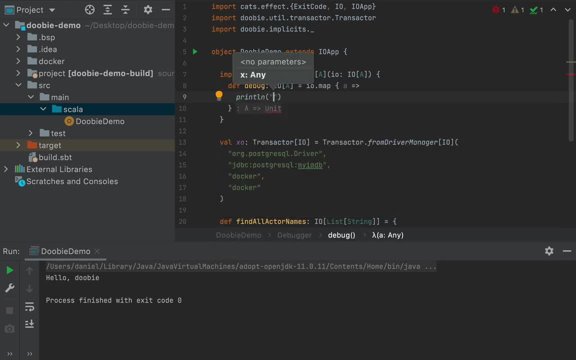 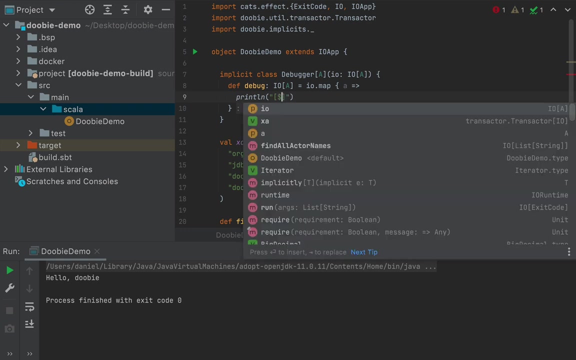 to print. so I'm going to say print line and I'm going to decorate that with the thread that ended up evaluating that, that IO, just to give you some insight on how these things will actually happen on top of the thread pull on which they run. So I'm going to run my little interpolator. 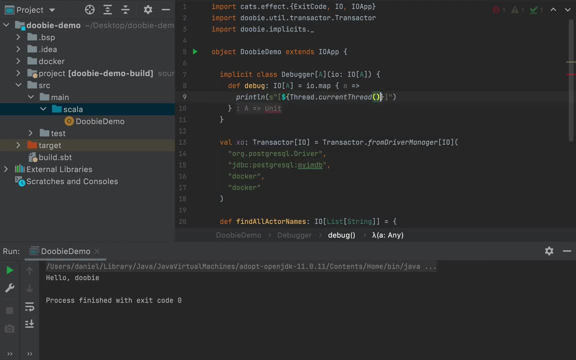 here I'm going to say threadcurrentthreadgetname and then, finally, I'm going to print my actual value and then I'm going to return the same value for the IO to be further mapped or processed along the way. So this implicit class is only for the debug extension method. if you're running skull 3. 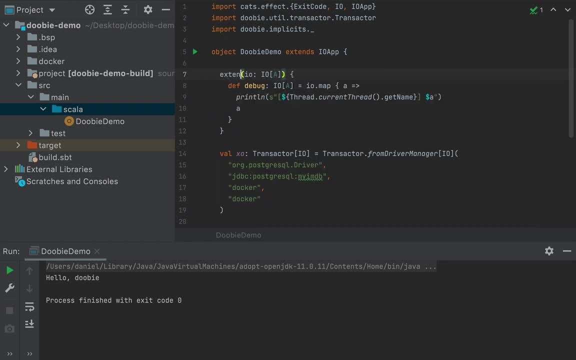 all you have to do is remove that. So this implicit class is only for the debug extension method. if you're running skull 3, all you have to do is remove the implicit class and just write extension. Now, of course, I'm using skull 2 in this project, so that 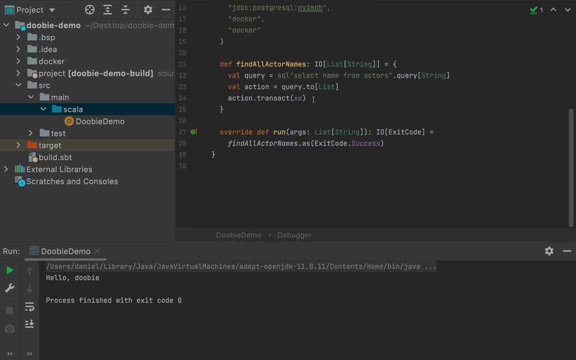 will now work, but otherwise that structure will run the same way. Cool, now find all actor names. I'm going to now decorate with my debug method because I now have access to that and I'm going to shamelessly run my application and I should see all the actor names that I have in my database. so 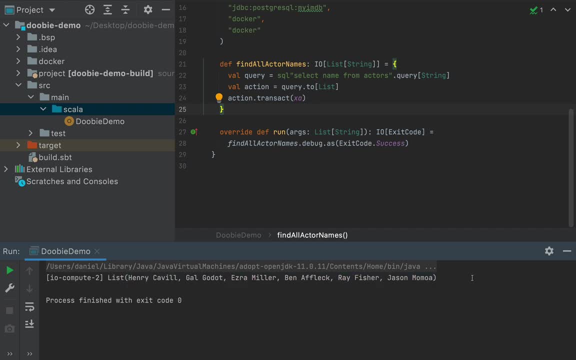 have list of, and then we have an actual list of actors from the database. so this is our start with the doobie library. that I want to show you is how do extract a single value out of a query if you want to select a particular name: a. 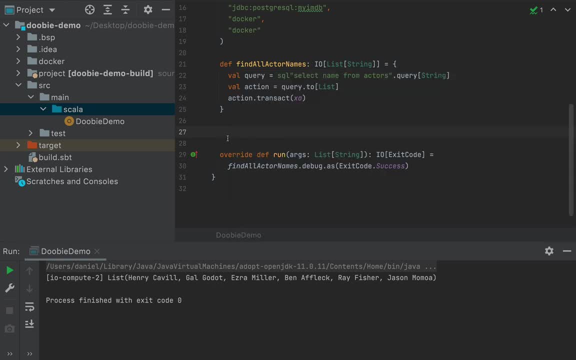 particular actor name from a particular ID. you can do that and return not a list of string but an actual string or an option string if that particular value is not present. and to that end I'm actually going to refused the supuesto in one cell but it didn't do out of account because I've never learned enough in the crash scene before. 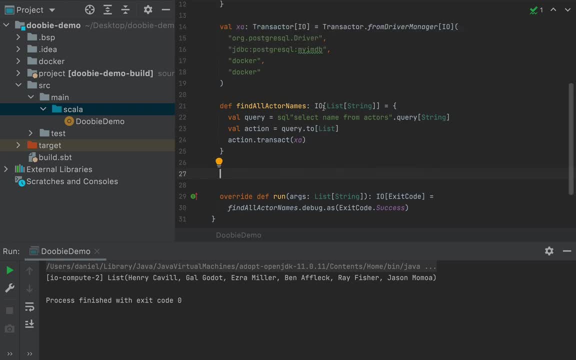 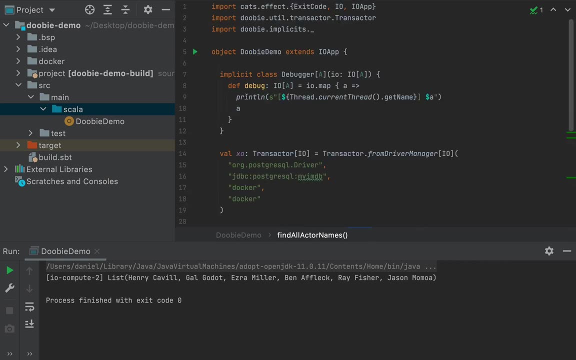 and to that end, I'm actually going to create a string name, some case classes, because we don't necessarily operate just with strings or ints or whatever. we also work with our own case classes. so I'm going to define a case class. I'm going to call this actor with an ID as an int and the name: 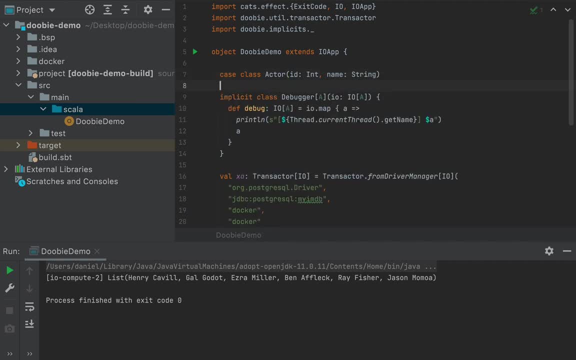 as a string, and I'm also going to create another case class. I'm going to call this movie and this will have an ID of type string, a title as a string, a year of launch, which is an int. actors, which is a list of string. this is the actual. 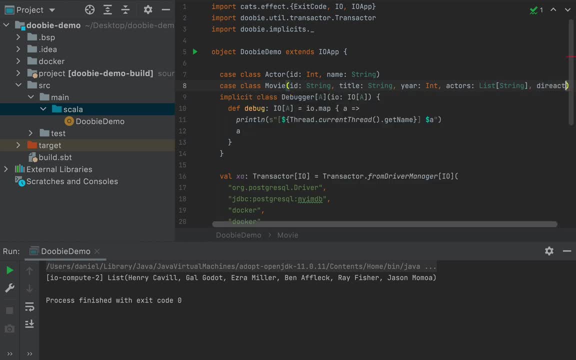 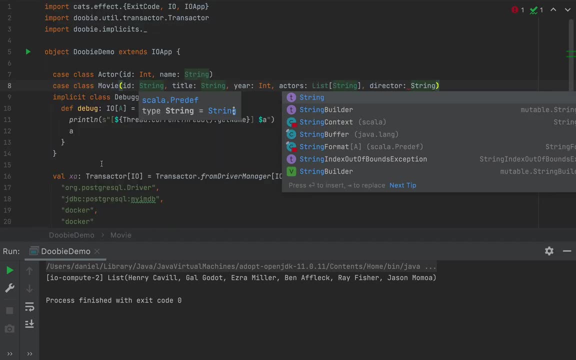 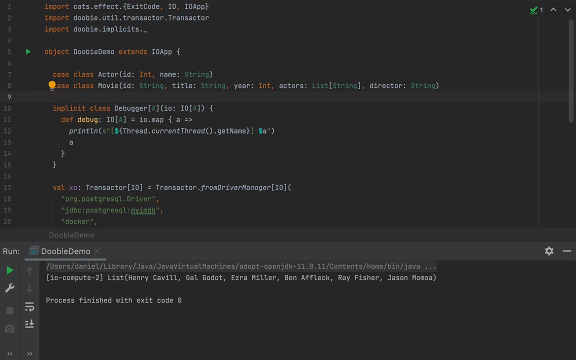 actor names, really, and the director direct, or which is a string. and my code is getting a little wide, so let me collapse my Explorer and that is going to be my other case class. now let's say that I would like to create, or rather return, the only actor for a particular ID, so I'm going to define another. 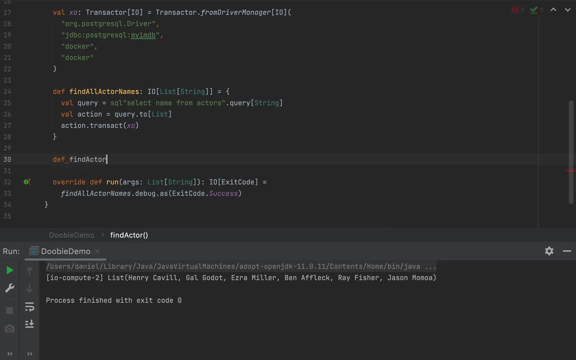 method and I'm going to call this actor with an int. and I'm going to call this method, let's say, find actor by ID, which is an IO of actor. now I'm also going to pass an actual argument to this method. let's say the ID which is of type int. 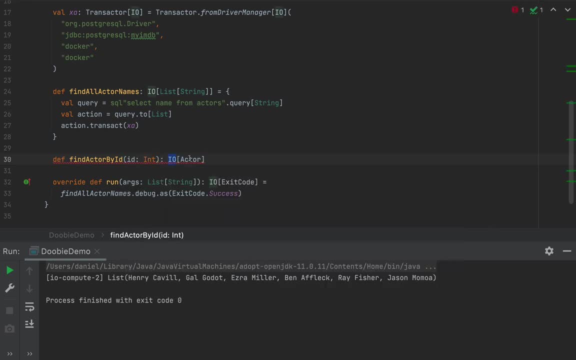 and this will return an IO. that is an effect which, when evaluated, will produce an actor. now I'm going to run the same pattern by first specifying the query, so I'm going to have, let's say, SQL quote, I'm going to say select ID name from actors where ID equals, and I'm 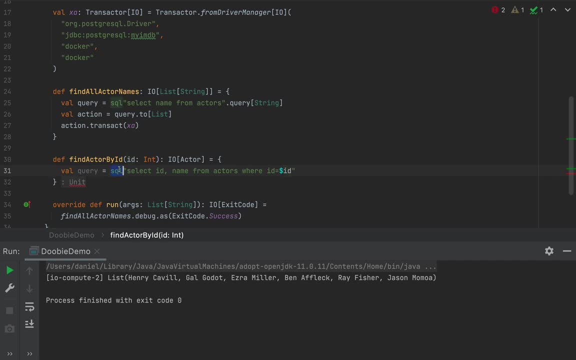 going to inject my ID argument. so interpolation has its own benefits, which is that you can inject the actual parameters directly in the query and I'm going to say query and now, instead of string the type, I'm also going to use the actor type. so query of type actor and. 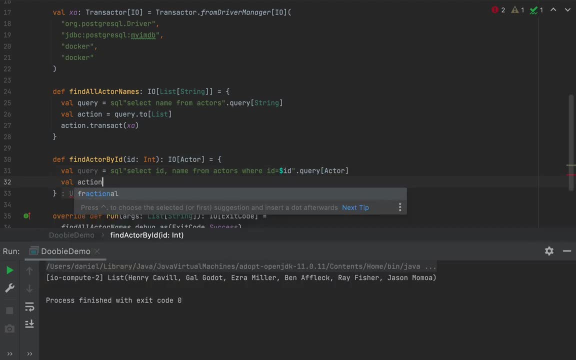 then I'm going to say, let's say action. I'm going to say query dot unique. query dot unique will return an actual actor and if that particular actor does not exist in the database, then this will throw an exception and you can then say action: Dahl transaction. 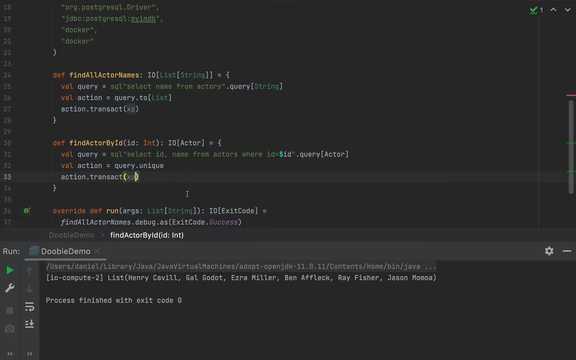 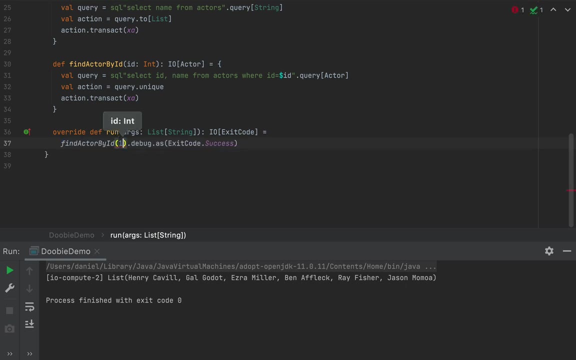 through that transactor X, a and we can actually call that. so I'm going to say a find actor by ID with, let's say, ID 1, debug, as exit code. success, and let me run this application. we're gonna see mister Henry here- this is going to be our actor- and notice that. 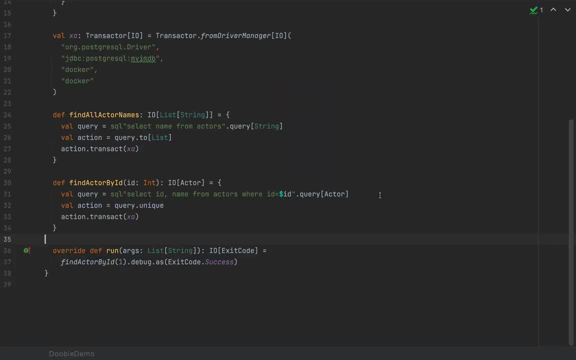 the conversion to our little case class happened automatically. now, if you're not really sure whether the actor exists in the database or not, you can use option. for instance, if I see find actor by ID, let's say use ID 99- then when I want to evaluate this, 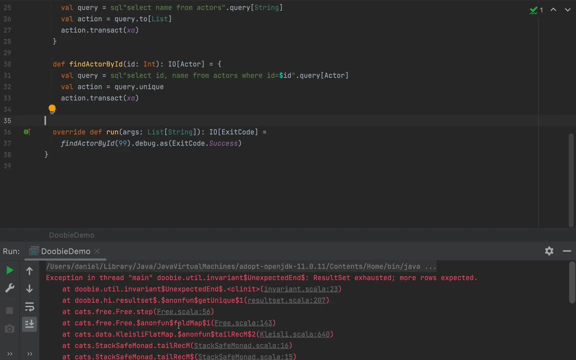 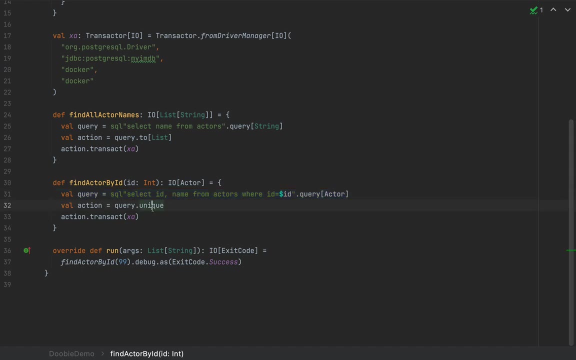 effect. it will throw an exception so you can see a stack trace: more rows expected. that is because we return the query actually returns 0 rows and I expect 1. if you are not sure whether that ID exists in the database, you can use option, but in this case the effect will return an IO of. 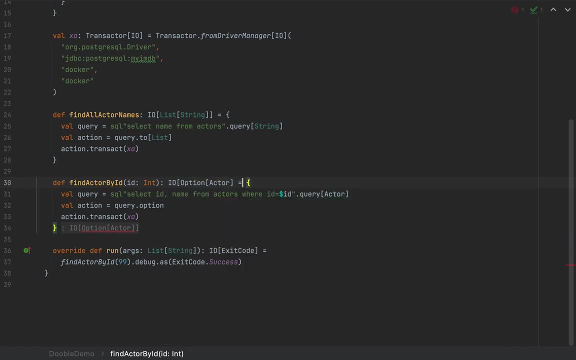 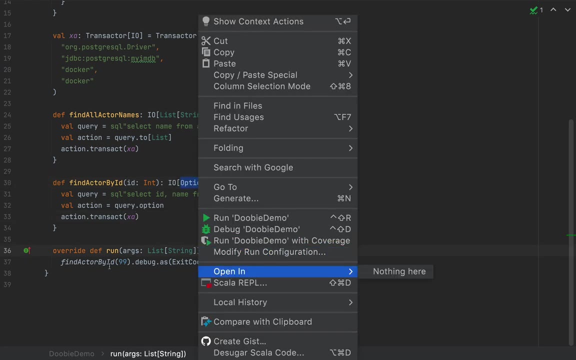 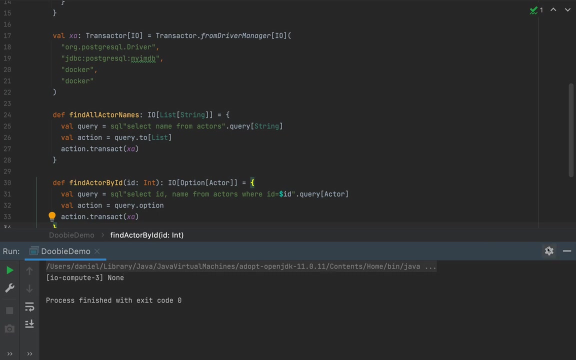 option actor. so I'm gonna say option actor in this case, and you'll be able to map that particular option when you evaluate that effect. so find actor by ID. 99 will return a none, right, cool. so that is how you can return a single value out of a query, either by saying unique or option. if you're not sure. 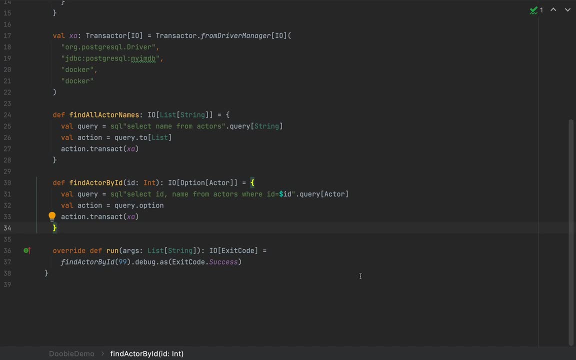 whether that query will actually return a row. cool. now, in practice, using a concrete type such as theひ lists of strings when you want to return multiple values is quite impractical and, frankly, quite dangerous, because if your tables are quite big, the lists might become quite big, And that is why 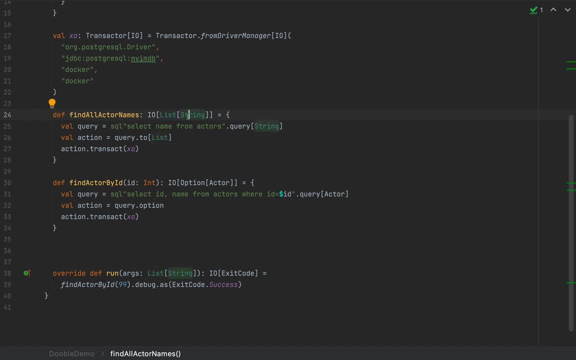 we tend to return multiple values as a stream instead. Now, because Doobie works in the type level ecosystem with cat's effect and such a stream is actually expressed as an FS2 stream. So FS2 comes from Functional Streams for Scala, FSS, also known as FS2, which is outside the scope. 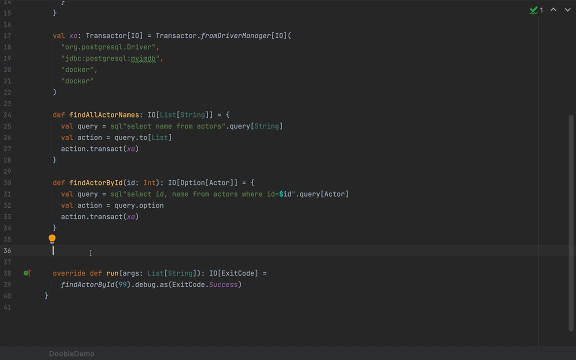 of this tutorial. We're going to have another tutorial incoming at some point And I'm going to demonstrate something very short. Let's say you want to return all the actor names as, not as a list but as a stream. I'm going to return actor names, stream as SQL quote and I'm going to say select. 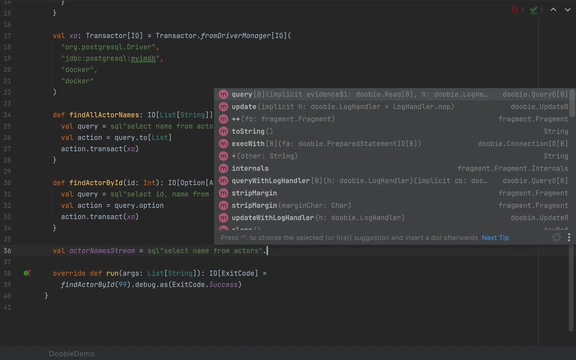 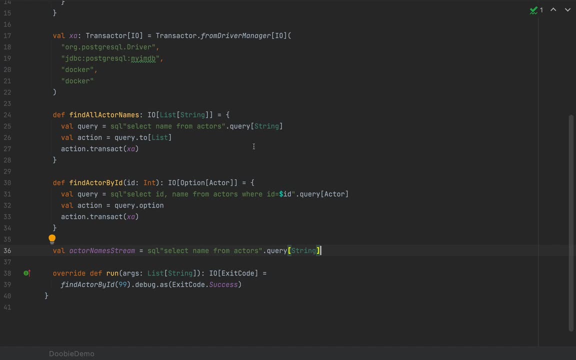 name from actors. And then I'm going to say query of type string, because these are the values that I'm after, And instead of saying queryto with a type list, I'm going to say dot stream. Dot stream means that I'm going to return a stream of and the resource type is connection IO, which is an. 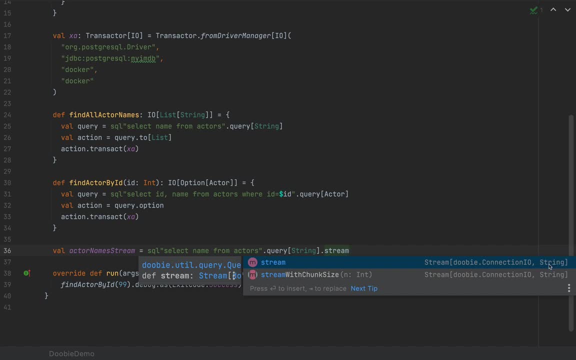 effectful connection to the database And the values that will pass through that stream are of particular interest. Now, if you want to actually turn that stream into a list, if you want to fetch all the items one by one or many by one, you can say dot, compile, dot to list, transact, And then 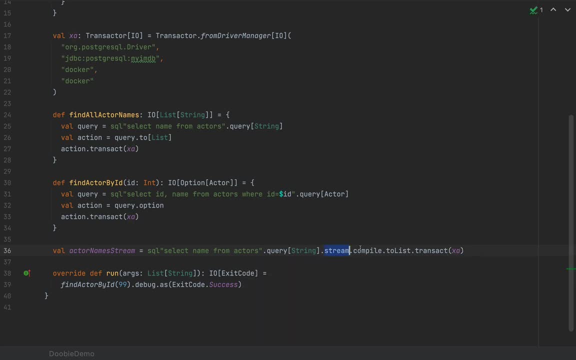 you can use that transaction manager XA, So the stream will actually be the definition of all the values that will be fetched at some point when you want to evaluate that stream. And then you can evaluate that stream by saying compile to list And this will collapse that string to an in memory. 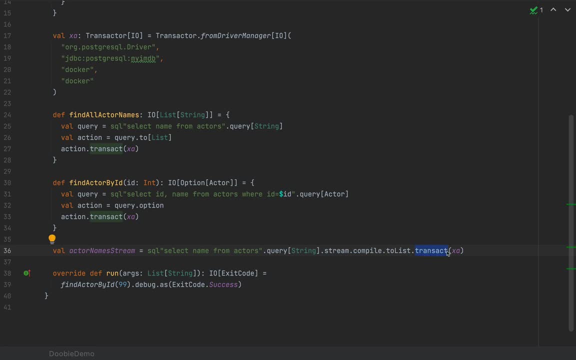 list And then this will be an effect which you can use, the transact with that particular transaction manager. So when you say to list, you'll get an effect managing a connection, And then you can call transact on that and you can pass in that transaction manager. Now this seemingly one liner will 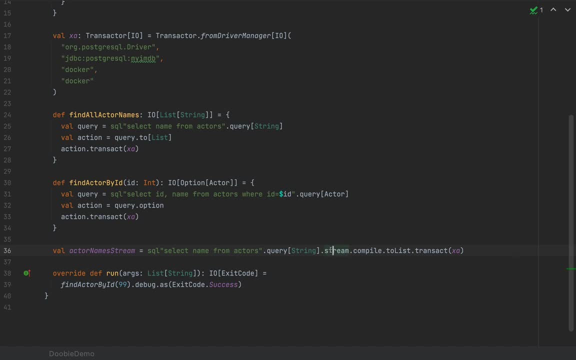 actually do quite a lot of magic under the hood. As you probably noticed, the goal was to use stream to memory. Now, of course, in order to prove this example, I brought the stream to memory, but that's not necessarily what you absolutely need to do. So if I'm interested in doing that, I can say: 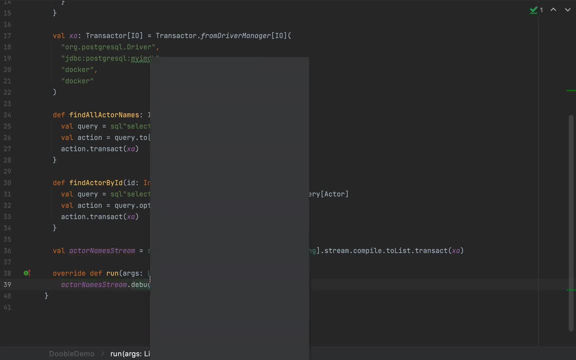 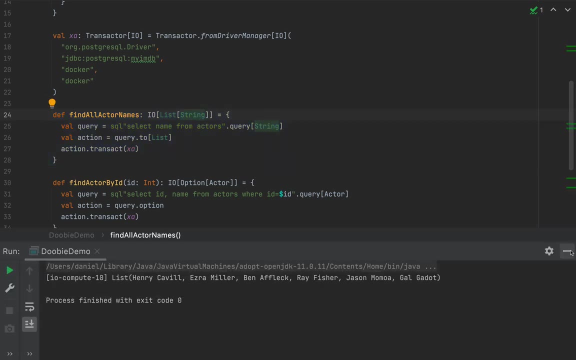 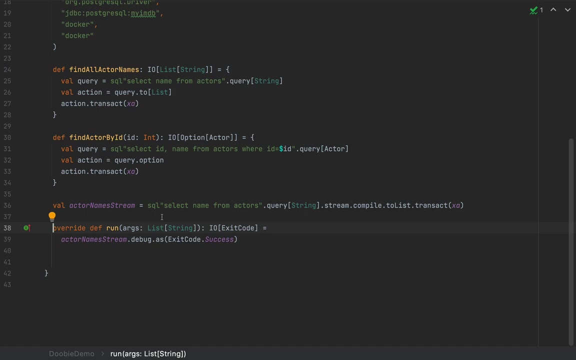 actor stream names, dot, debug as exit code success And we are going to see the same results as the original query. All right, so we have all our little actors- Amazing. Now, folks, these are the high level ways of querying a database. there are lower level things which you can use. 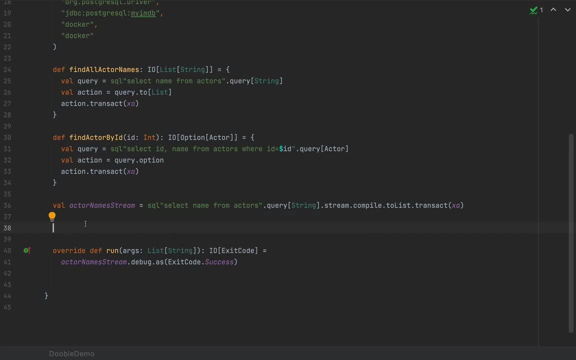 which give you a crazy amount of control, but they are also proportionally difficult to use And, quite ironically, they're still called high level connection, or HC and HPS for high level prepared statement. And I'm going to demonstrate a similar query such as this one which returns a stream And let's say I 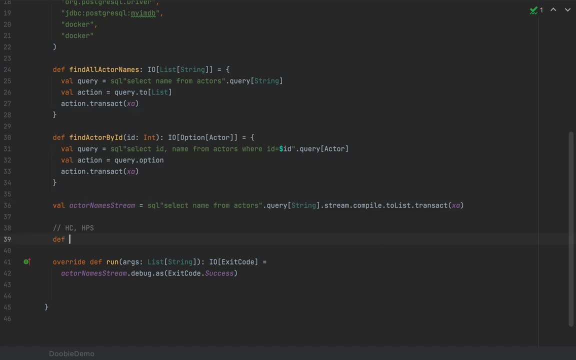 want to find an actor by their name. So I'm going to define, let's say, find actor by name, And I'm going to pass a name as a string And I'm going to return an IO of option actor And I'm going to run my little query as a string. So I'm 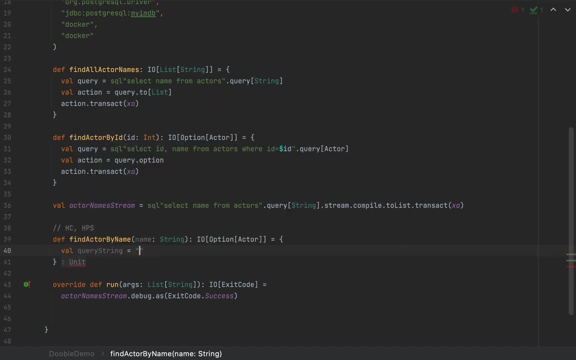 going to say query string as select ID name from actors where name equals, and I'm going to use a wildcard token here which doobie will parse eventually, And I'm going to say HC and I'm going to import HC from. 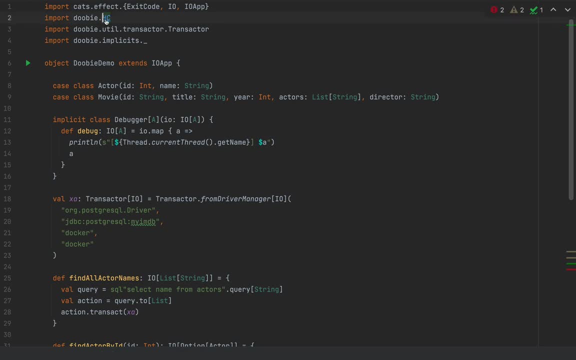 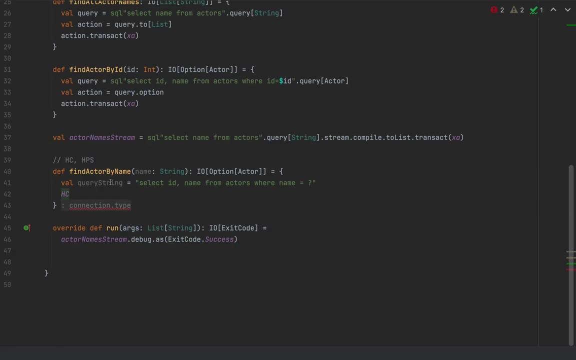 doobie. So this is doobie dot HC, which is an alias for high dot connection. This is an object with some API's, So HC for high level connection. I'm going to use HC dot stream And we will need to pass the actual type that we're. 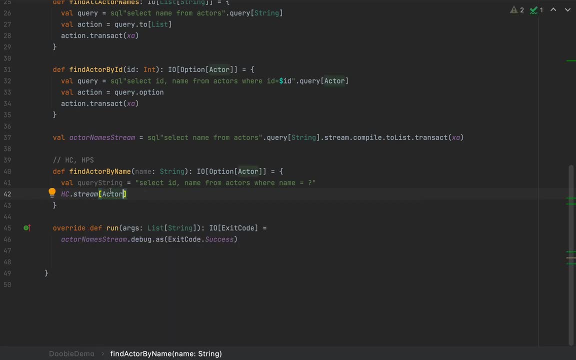 expecting. So these are the values that we are going to return when the query is being evaluated, And I'm going to pass a bunch of arguments here. So I'm going to use query, the query string, And I'm going to use a prepared statement, which is a bunch of 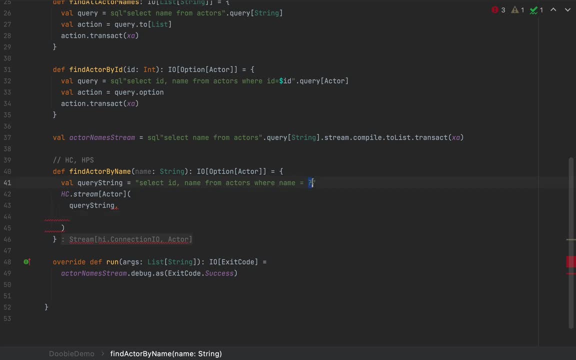 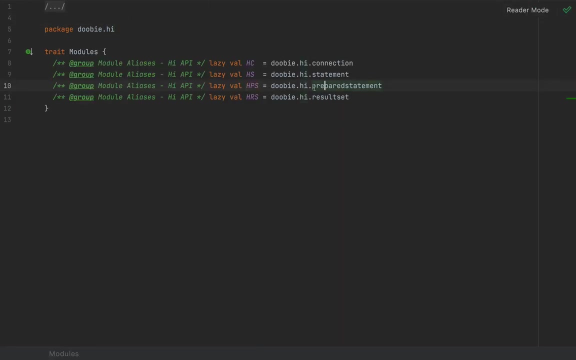 arguments that doobie will then use to replace these wildcards with, And to that end, I'm going to use HPS, which is another module in doobie that I'm going to automatically import. So we have doobie dot HC and HPS is a prepared statement, again an object with a bunch of APIs, and I'm going to use HPS dot set. 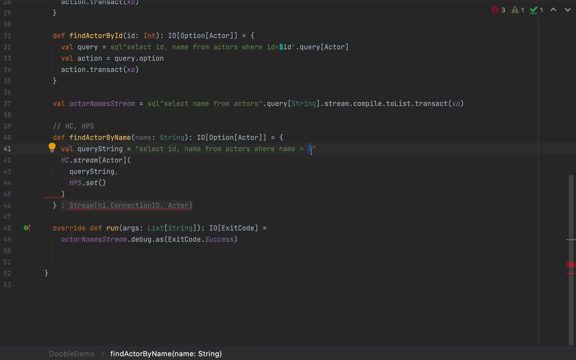 to set my little argument that I mentioned earlier. doobie will replace the wildcard with. So I'm going to set the name here as the first argument for the wildcard and then the chunk size for the stream, because doobie will read values in chunks, not all at once. I'm going to use, for instance, 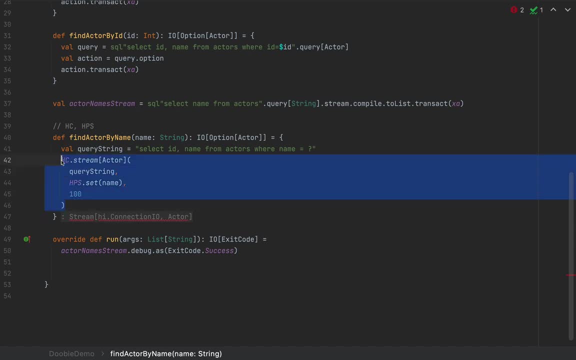 100 elements at once. Now, so far, this is a stream, an fs2, so we're basically up to this point. after calling stream, Now I'll need to say compile, and then I'm going to say to list, and then, if I get, 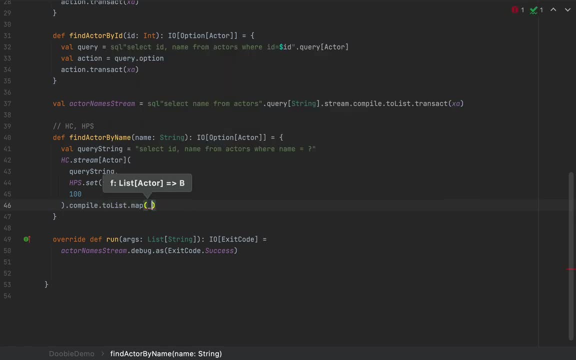 a list, I'm going to say map and I'm going to use head option to return the first actor whose name is equal to whatever wildcard I use here. So up to this point we have that connection IO thing which I'm going to use to say transact on that transaction manager. 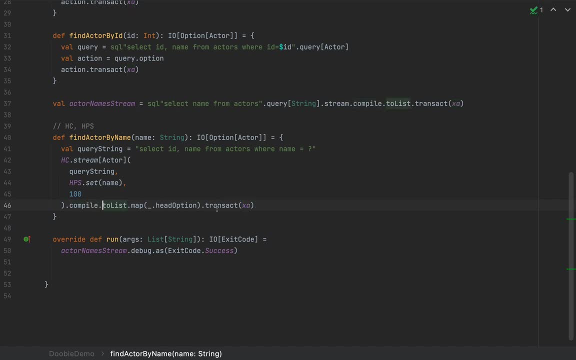 or transactor. So the compile to list transact xa is the same as the last part of the actor name stream example. Only that in this case we used a lower level API which managed the query string manually, the parameter list manually and the chunk size manually for the stream. So if I say 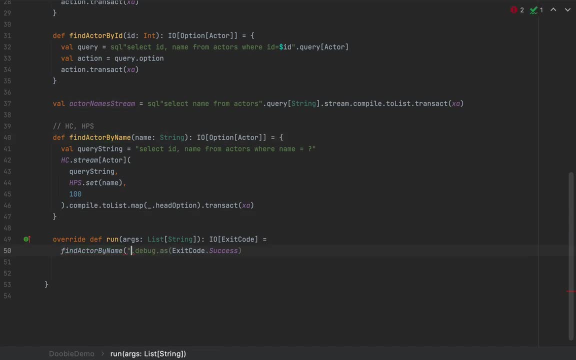 find actor by name with the name Henry Cavill, if I remember the name correctly. If I run this application, we're going to see that particular actor. Alright, so we have actor with the ID 1, Henry Cavill. Okay, so that was an option with a lower level API. 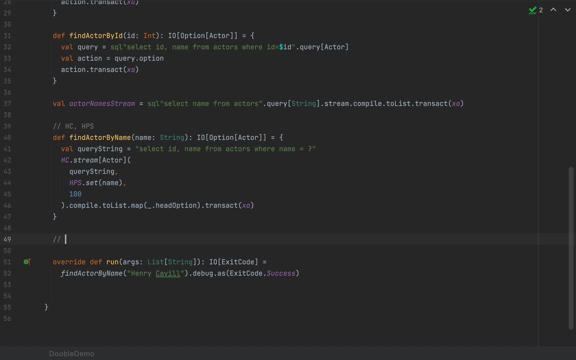 using HC and HPS. Another lower level API is fragments, which means that you can define variable pieces of queries that you can then combine into one. So that is, if you want to automatically generate queries by yourself, these fragments are a good way of doing that. 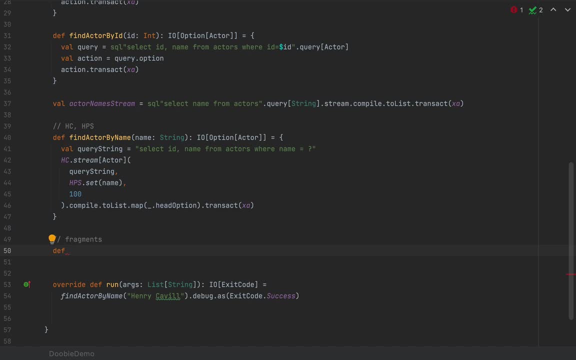 So I'm going to run another example. I'm going to say find actors by initial letter, for instance. I'm going to say find actors by initial letter, and I'm going to say letter as an argument, as, let's say, a car or a string doesn't really matter all. 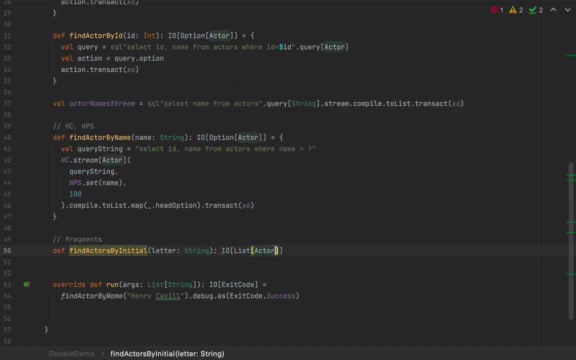 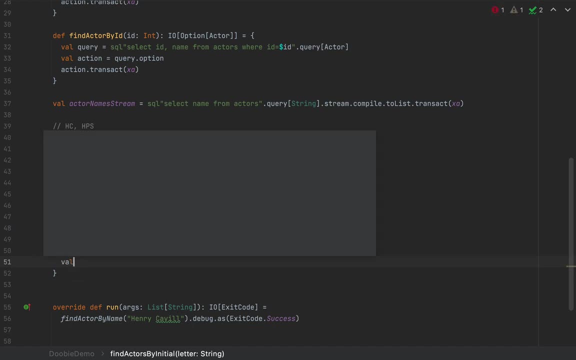 that much and I'm going to use an IO of list of actor as my return type. cool, now you can define variable pieces of queries and, for instance, if I want to split my query, select ID name from actors where initial letter equals whatever, I can say the select ID name. this is a fragment, let's say the select. 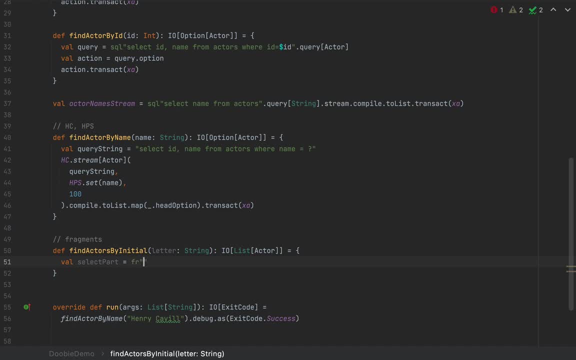 part as fr quote. this is another custom string interpolator which do we supports. fr comes from a fragment, of course, and you can say select ID and name, that is, if you want to generate the number of columns that you want to select from the database. you can do that and I'm going to have the from table, the from part as. 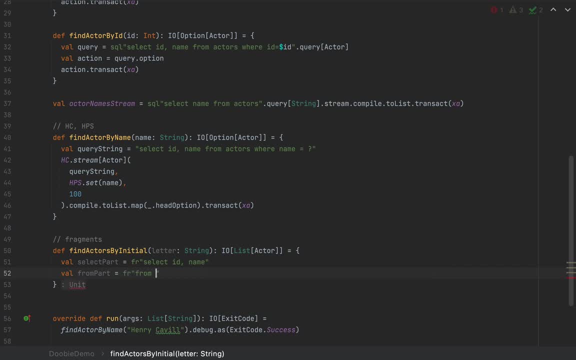 a fr quote from actors, actors, and then I'm going to use the filter or the where part as fr quote where, and I'm going to use left with name and one that is the first letter of the name column must be equal to, and this is where my string. 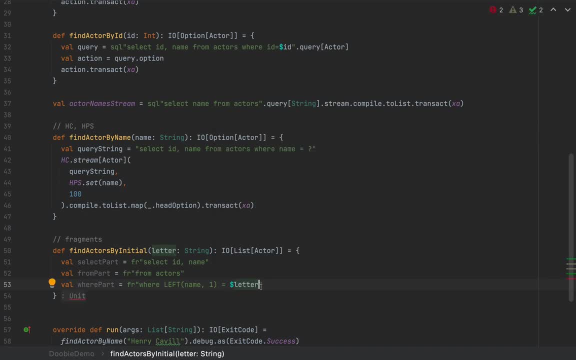 interpolator is doing its magic. I can inject here and that I can combine all these parts to combine a single statement. so I'm going to say: is a cell query as an, I can use select part plus plus from part plus plus were part, so you can combine all these fragments into one statement. 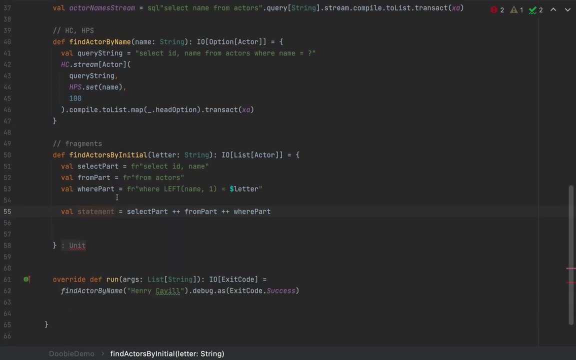 I'm actually gonna call this statement because in order to turn that into a query, you'll need to call the query method on this. so it would've been pretty weird if I said queryqueryActor. so I'm going to say statementquery of type actor and then you 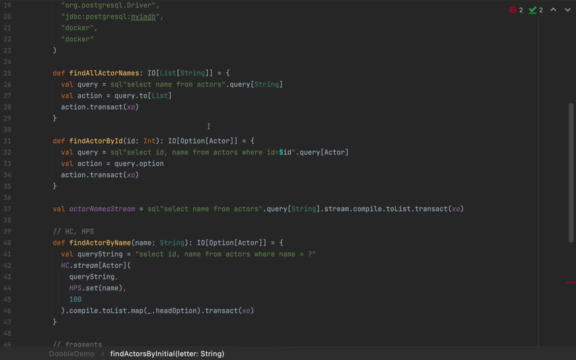 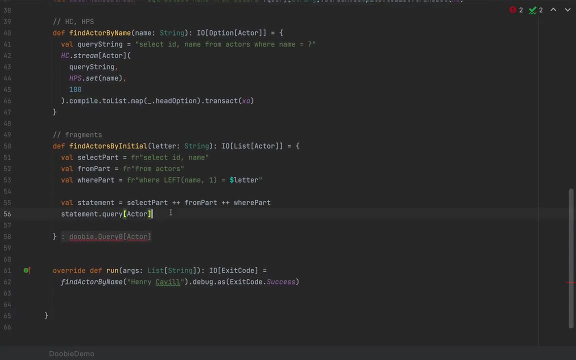 can use the other continuation that you learned from the previous example. So you can say query to list query, stream, compile to list, transact, whatever. You can say anything that you like. So I can say streamcompiletoList transact and I'm going to use that. transaction manager xa. 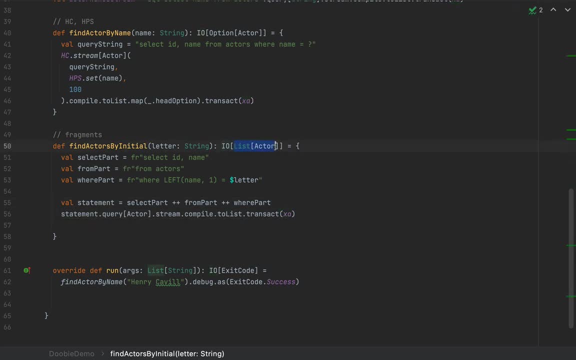 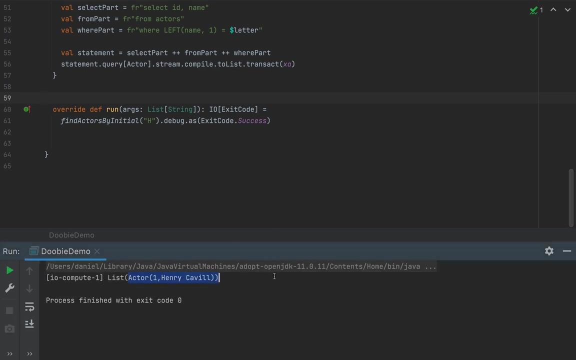 All right, so this will be an effect which will return a list of actors. once done, So, find actors by initial, and I'm going to use the letter h because it's really easy and we're going to see at least Mr Henry returned in my final result. All right, so these fragments are a very useful 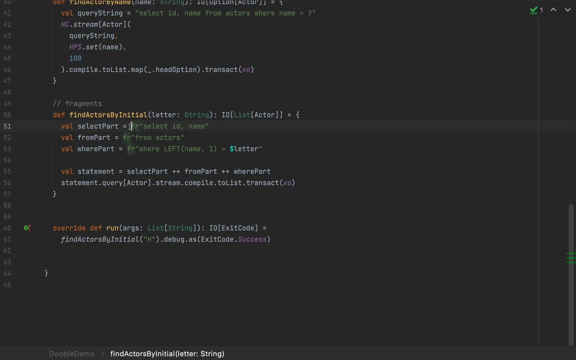 tool for generating queries automatically or programmatically, by generating pieces independently And then combining them all together. Now the written version of this tutorial. the blog post has a bunch of tips on how to use the monoid syntax with these fragments, if you're interested. 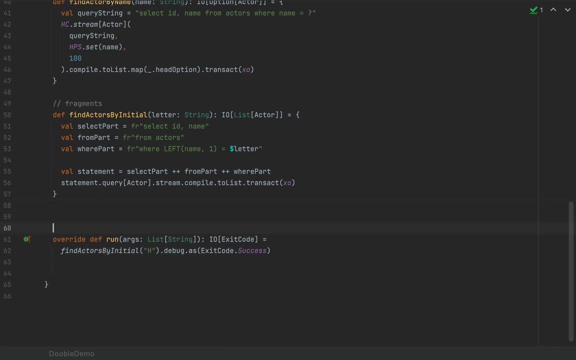 in that sort of stuff in cats. Now, another thing that I wanted to show you was how to update stuff into a database. For instance, if I want to save an actor into my database, I would run the following thing: I'm going to define a method, say save actor. 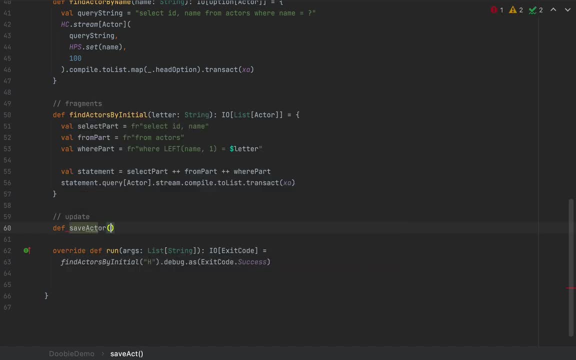 And I'm going to have an ID as an int and the name as a string And this will return an IO of int And this will be an effect which will contain, when evaluated, the number of rows affected. All right, Now I'm going to define my little query, So I'm going to have query as SQL quote. 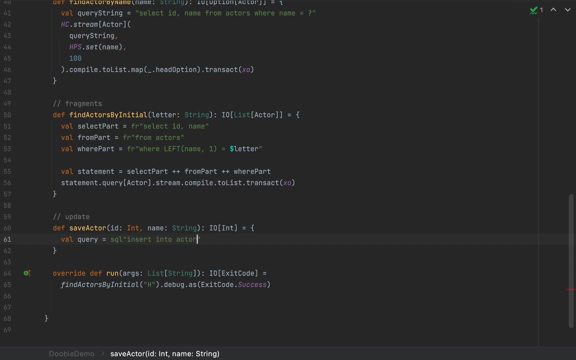 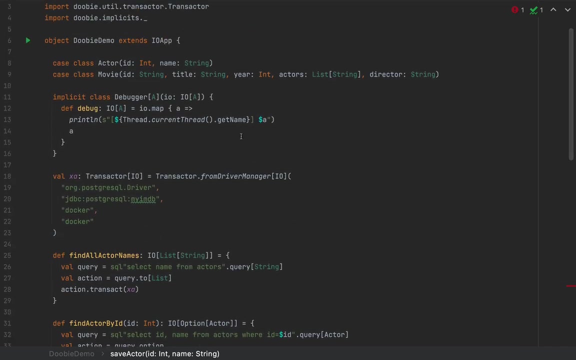 and I'm going to say insert into actors and I'm going to have the title, ID and name values and in parentheses I'm going to have ID and name taken. Now I'm going to say query And instead of saying to list or whatever we did earlier when we fetched items from the database, 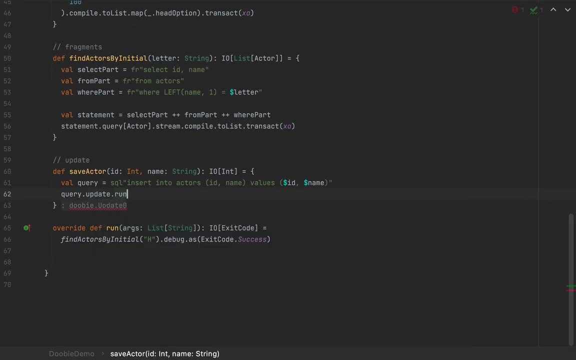 we can say queryupdaterun And then I'm going to have transact on that transaction manager. so query update, run. this is a connection. i o returning the number of rows when that particular query is executed, and then i'm actually going to run that and return an effect with the transact method, as we did before. 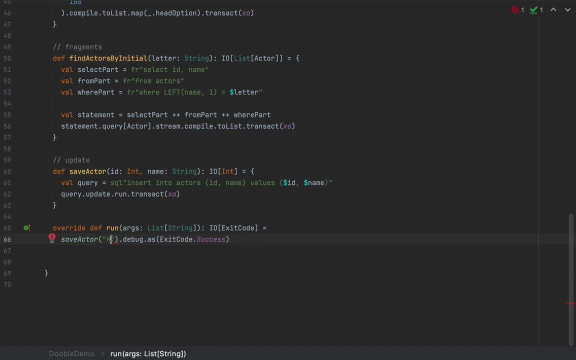 so let's say i want to call save actor with the id, let's say 99, and this will be an int and the actor name is my own name, daniel, and we'll have debug as exit code, dot success. if i run this application, we will have number one here being 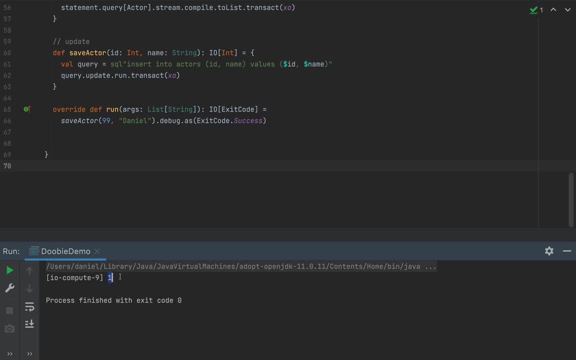 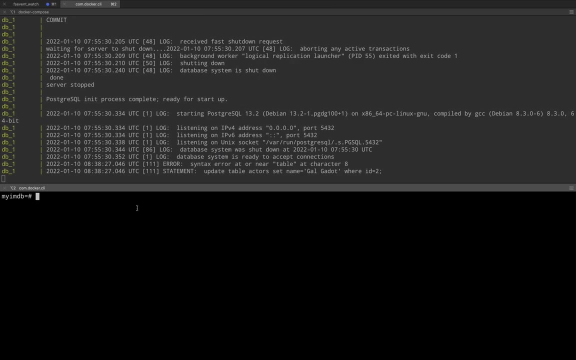 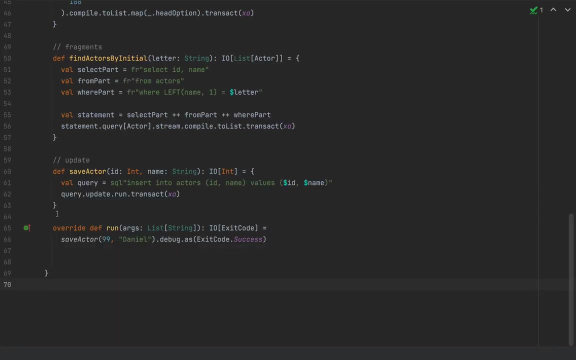 printed, so one meaning the number of affected rows, and the application exited successfully. now if i want to actually query the database, i'm actually going to say select star from actors and a colon, and at the id 99 i have my name here in the database, so i'm on the record. 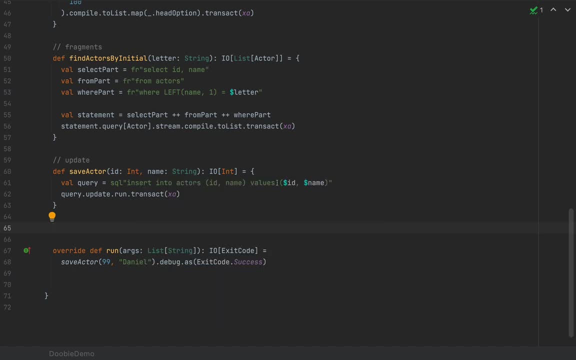 now you can also insert items into the database with auto generated id, so that you don't have to manage ids yourself. but only some drivers and some databases support that, and a query will fail if more than one row is being affected. so i'm going to show you how you can update with auto generated. 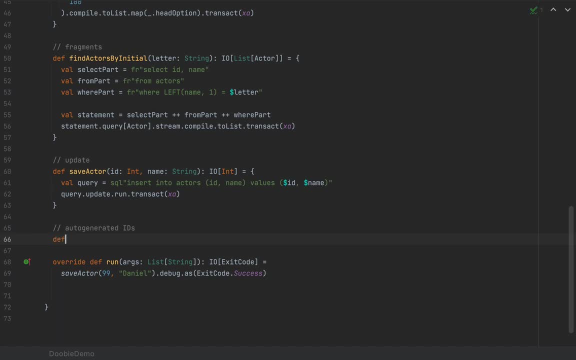 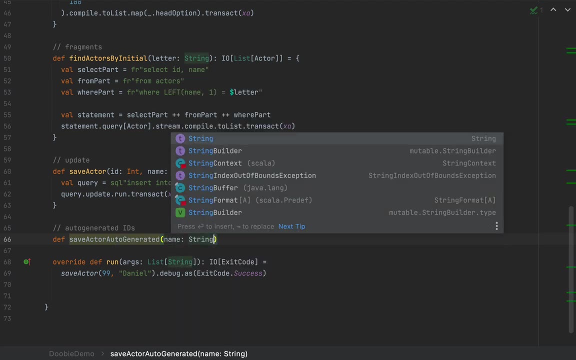 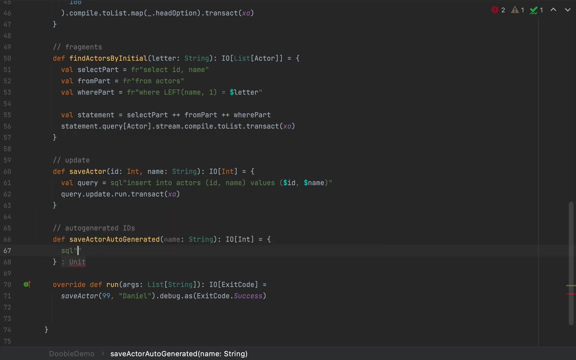 ids. so i'm going to say save actor auto generated and i'm going to have a name which will return another io of int and in this case the int will return the key that was generated. so i'm going to say um sql quote. i'm going to say insert into: 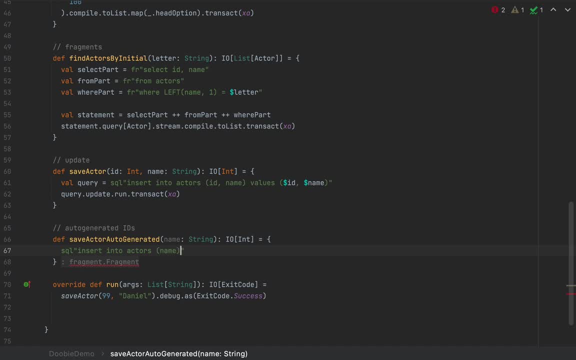 actors with on the column name and I'm going to have values and I'm going to, in parentheses, inject my name argument and this SQL query can be decorated. so I'm going to say update and then I'm going to say with unique generated keys and this will need the 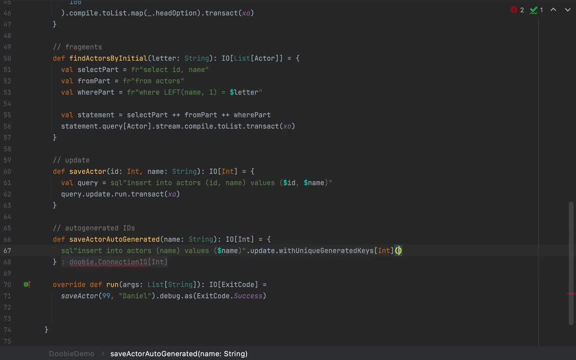 appropriate type argument for the column type and the column name for which we want doobie to generate the new key. and the column name is obviously ID here, cool. and finally I'm going to say dot transact on that transaction manager- cool. so I wrote this in a one line. now I'm gonna use the save actor auto. 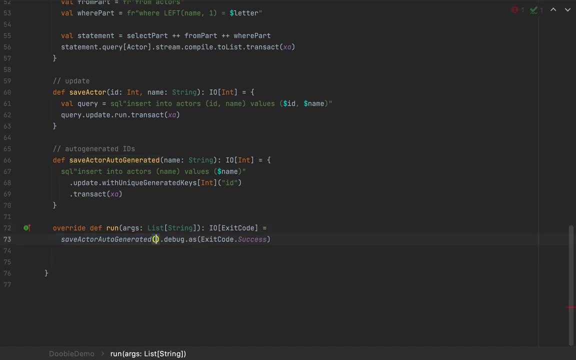 generated into the console and let's inject another name, let's say Jimmy. cool, now Jimmy is going to be inserted into the database and we're going to see something being printed to the console, which is the number 7. this is the first ID that could be uniquely generated by doobie, and here 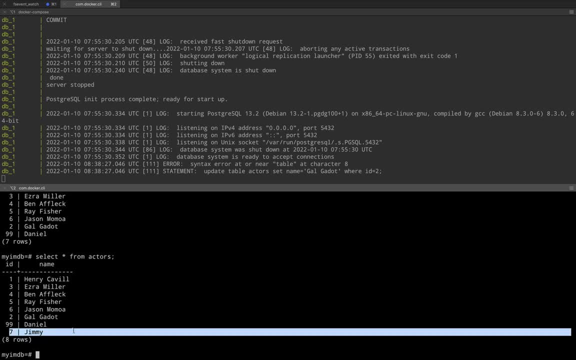 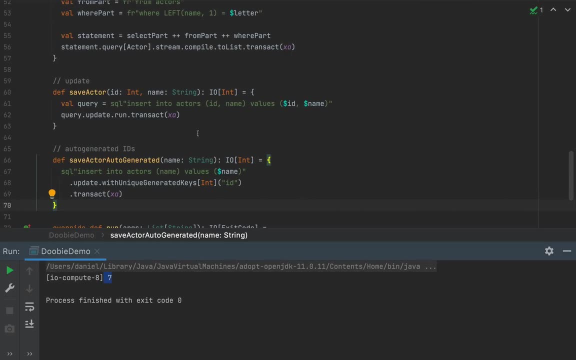 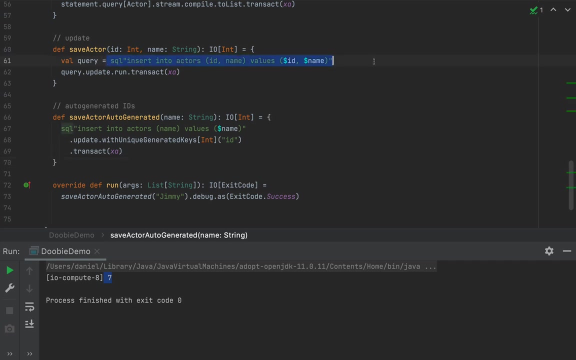 in the database, if I query select star from actors, notice that Jimmy was automatically inserted with the first ID that could be generated. cool, now there are a bunch of ways of expressing the same thing, because doobie is a pretty rich library. for instance, this sequel string, sequel insert into actors values. 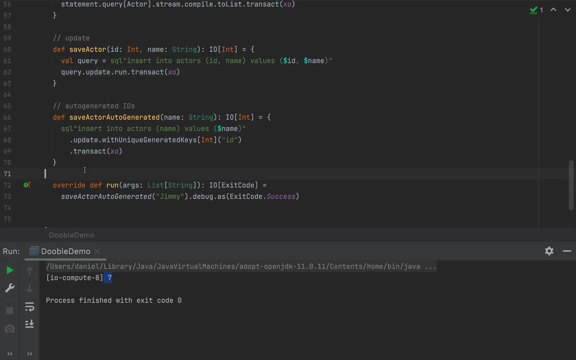 update. run transact is equivalent to another way of doing the same thing with some explicitly mentioned types in doobie. so I'm going to define a save actor version 2- with ID, type, int and name as a string. this will return io, int and I'm going to run my sequel string. so I'm going to shamelessly copy that. so I'm 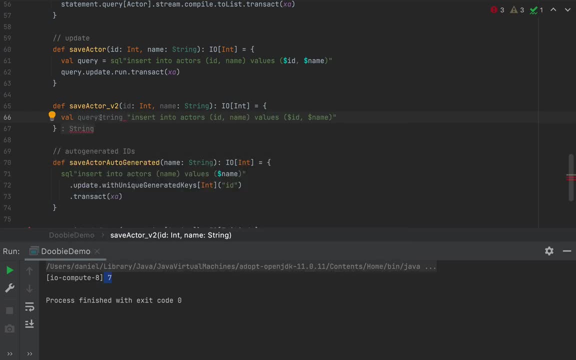 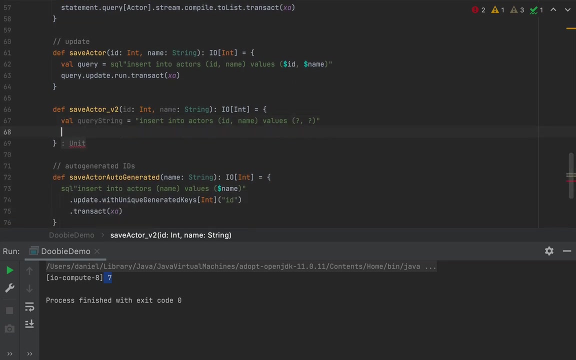 going to have query string right, so my query string is equal to the same string as earlier and instead of ID and name I'm going to use question mark and question mark- the wildcards that we saw earlier now, unlike the hc and hps kind of stuff that we saw in the previous example- we're going to use. 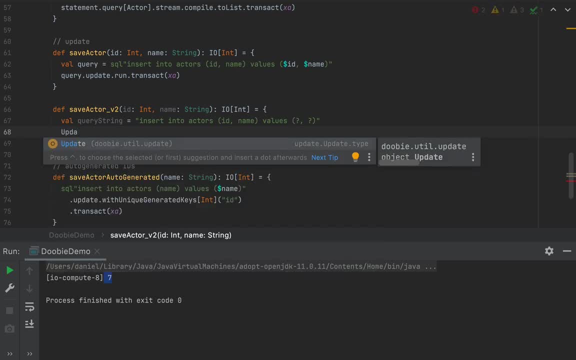 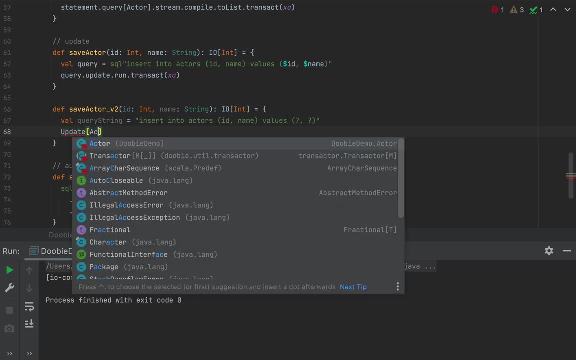 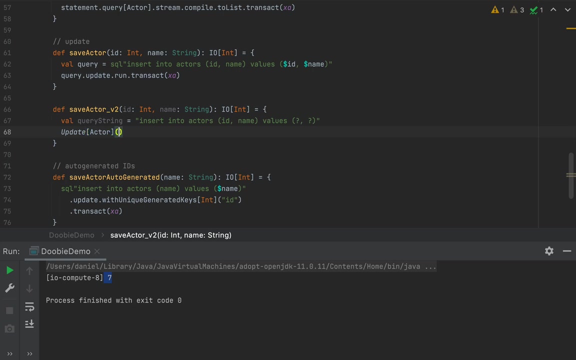 an explicit type called update that you need to import from doobieutil update. I'm importing this automatically, so I'm gonna say update of type actor, so this is the type that I want to inject into these values, and then I'm going to run the apply method on that query string or insert statement rather, and that. 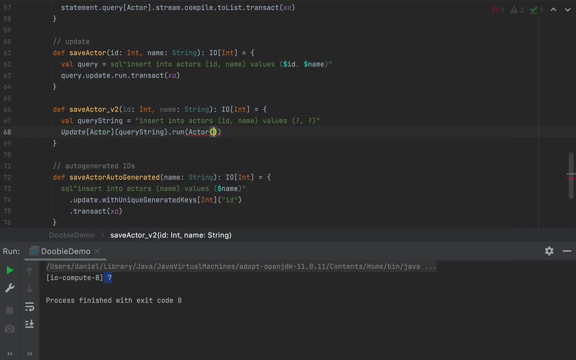 I'm gonna run on an actor, So I'm gonna say actor, with the ID and name that I receive as arguments to the method. Now this thing, this line 68, is equivalent to saying: query dot update. after running the SQL string interpolation. Now after: 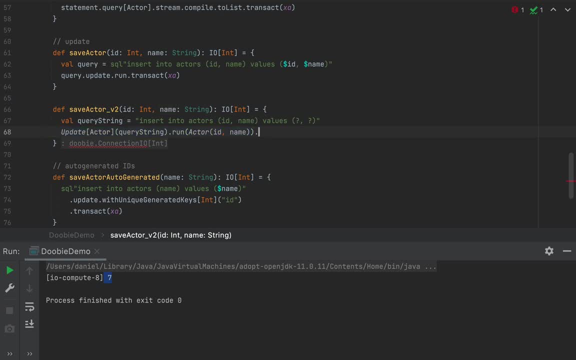 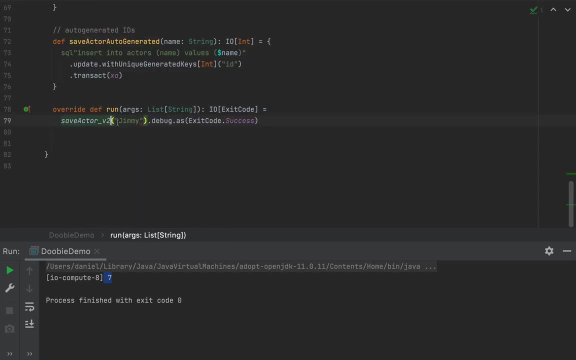 creating this connection IO, then I'm going to call transact on that transaction manager that we saw earlier. So save actor version 2 should work in the same way If I pass in the appropriate arguments. so that is the ID ace and I'm going to use, for instance, Mary. this should work in the exact same. 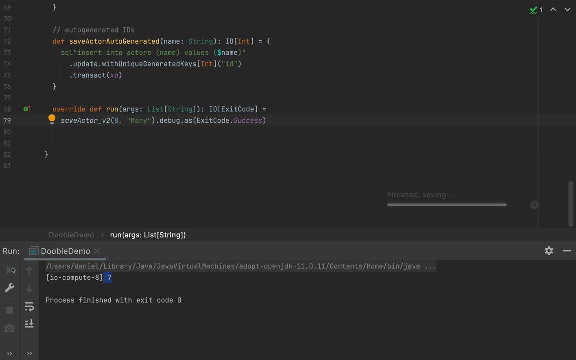 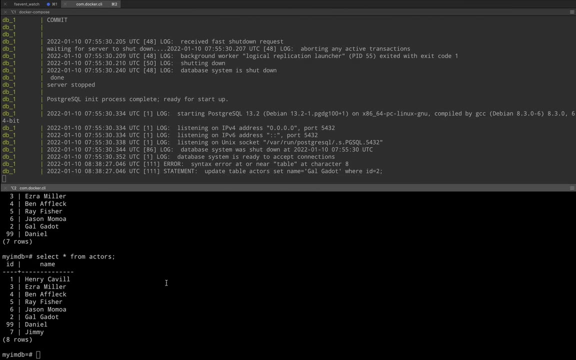 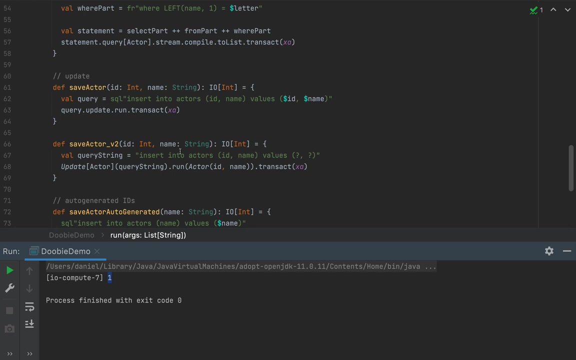 way as before. So let me run the application. and now. the number one means the number of rows that were affected by the insert statement, and my database should now show a new row, So the ID 8 and the name Mary as my actor. Alright, now this particular more. 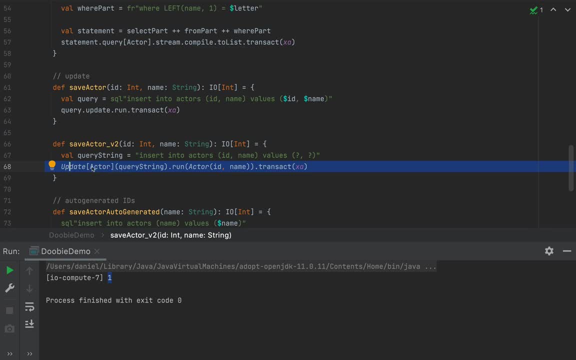 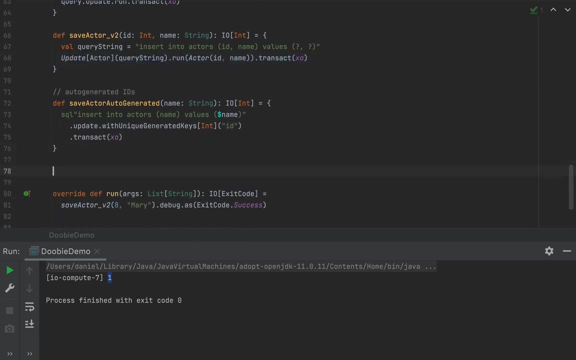 cumbersome way of running an update statement is pretty useful because this also allows us to run an update many kind of query, So when we want to update, or rather insert, multiple values into our table at the same time. So I'm going to show you: update many or insert many. 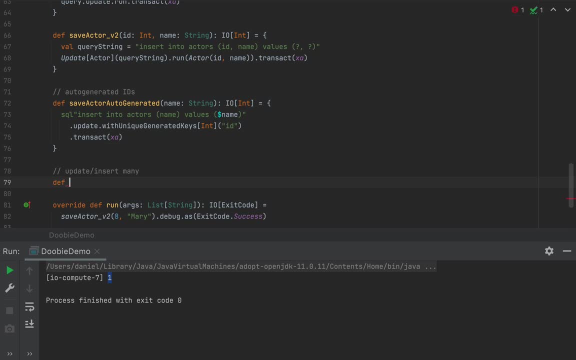 So for this example, I'm going to use, for instance, save multiple actors and I'm going to have the actor names as a list of string and this is going to be an IO of int. Now I'm going to use my insert statement. so I'm going to have my insert statement as. 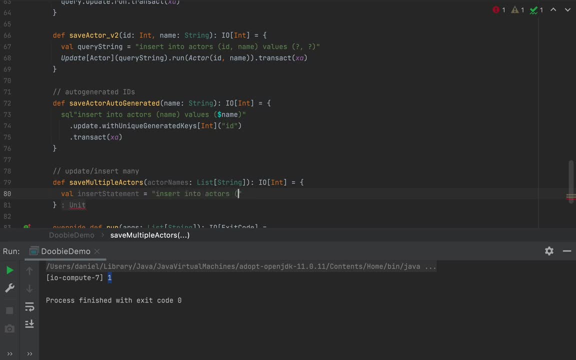 insert into actors where the column name is applicable to us values, and then I'm going to use a little wildcard. Alright, now my insert statement will be subject to an update query or data type or apply method, or however you want to call this, and I'm going to have update with the type string in this case, and I'm going 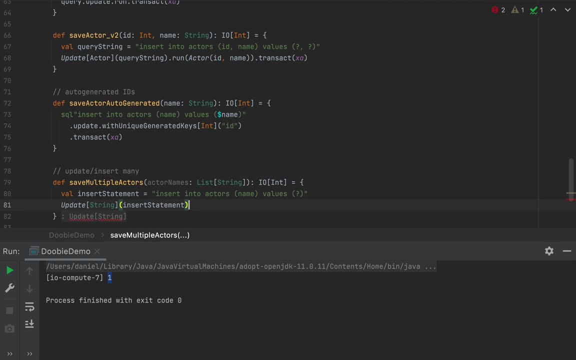 to pass my insert statement as a string and then I'm going to pass my insert statement and I'm going to use updateMany and notice that you can use updateMany and updateMany with generated keys, as we did earlier. Now updateMany is an effect that will return the number of rows that were affected. 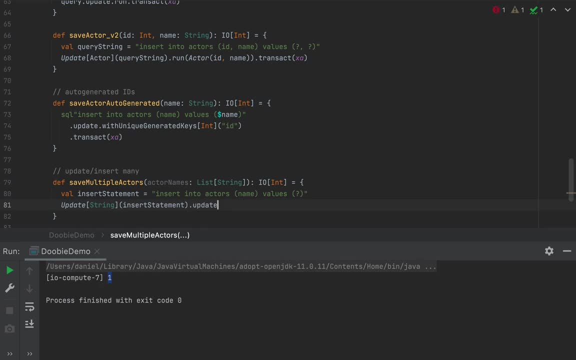 and for this particular case, I'm going to use updateMany with generated keys and, instead of returning an IO int, I'm actually going to return an IO of list actor that were also created by changing number of rows. and Ahhh, now I can use this Shaft key here. 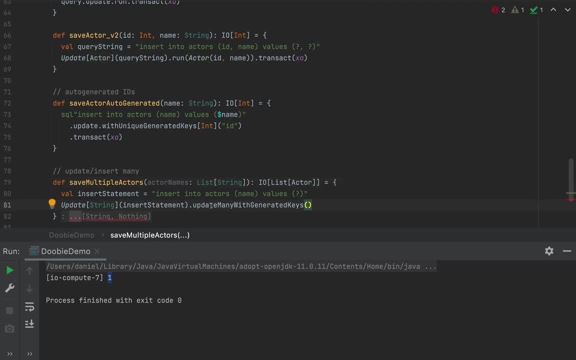 before updating the database. So I'm going to say updateMany with generateKeys And I'm going to type that with actor. So I'm going to help the compiler by passing the appropriate type And I'm going to pass the column names. So id and 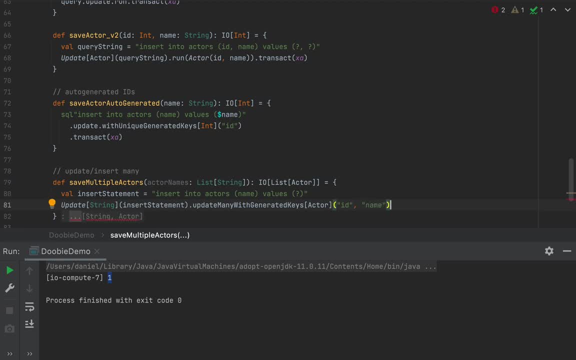 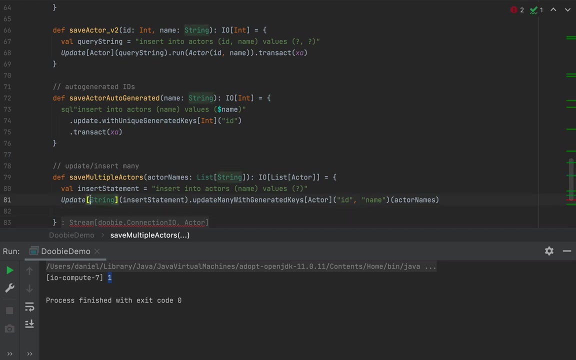 name And I'm going to, as an argument, I'm going to pass my actor names to replace that particular wildcard. So I'm going to say actorNames- Cool. Now, this particular statement is my updateAction. Now this particular updateAction is going to return if I'm 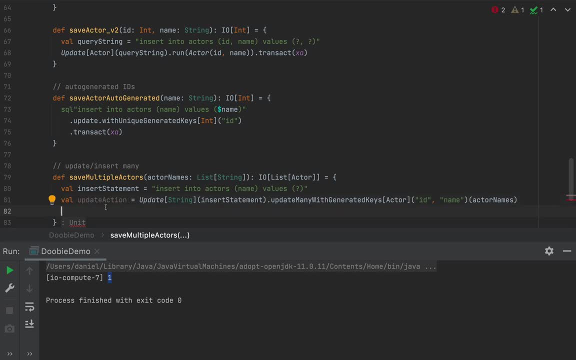 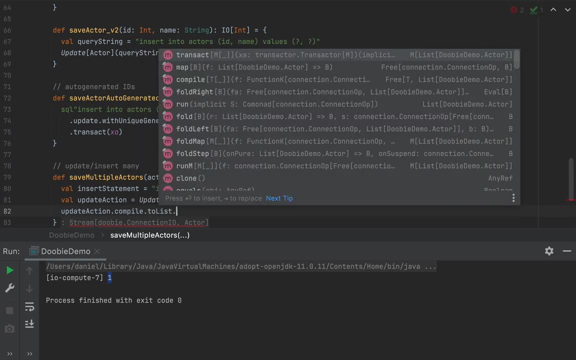 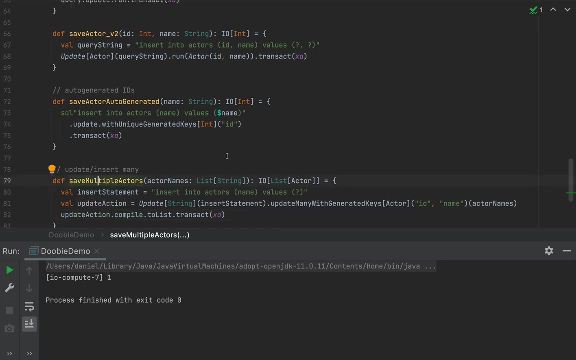 not mistaken, this is going to return an fs2 stream, So I'm going to return updateActioncompiletoList and then, finally, I'm going to call transact on that transactionManager, as we did earlier while managing fs2 streams. Okay, now, if we want to test this, we can call. 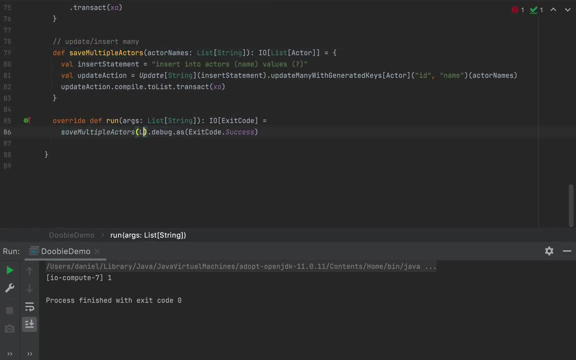 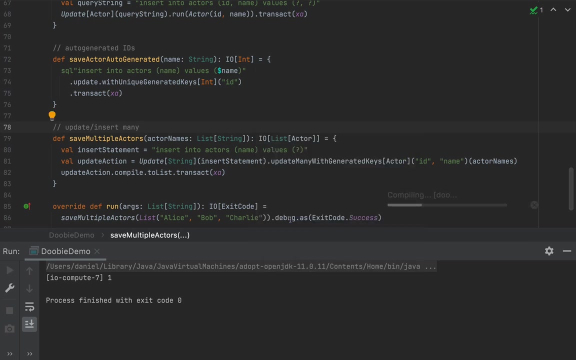 saveMultipleActors And of course I need to pass a list here. So I'm going to say list with Alice and then Bob, and then let's say Charlie, Debug as exit code: success, as before. Let's run this And we should see Alice, Bob and Charlie being 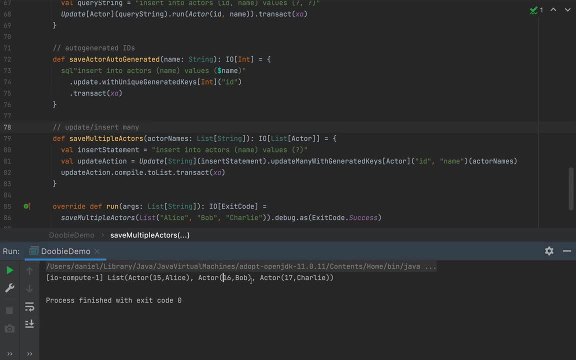 inserted into the database. So we have 15,, 16, and 17.. Not sure why the database generated these particular IDs, but whatever. And Alice, Bob and Charlie should be available in our little database. So select star from actors should. 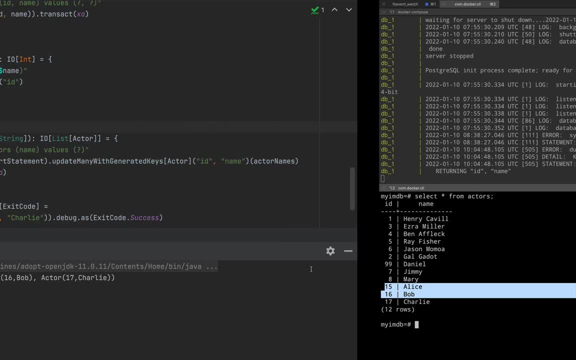 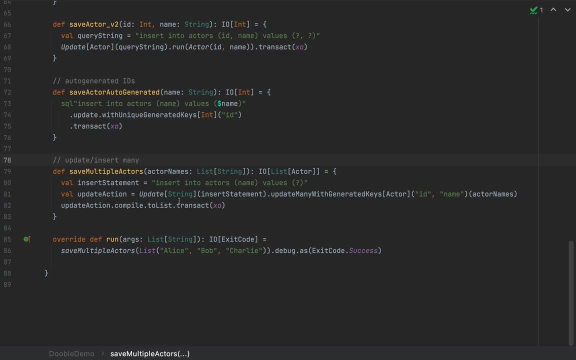 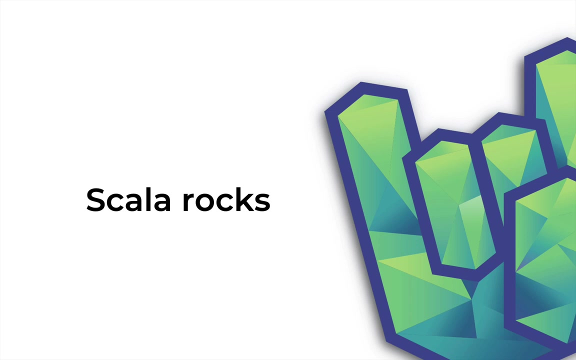 give us Alice, Bob and Charlie with these particular IDs- Amazing. So this is how we can insert multiple values at the same time into the database with a single query. So this was your introduction to Doobie. Now I have much more to show you on doobie, and the written version at the blog contains: 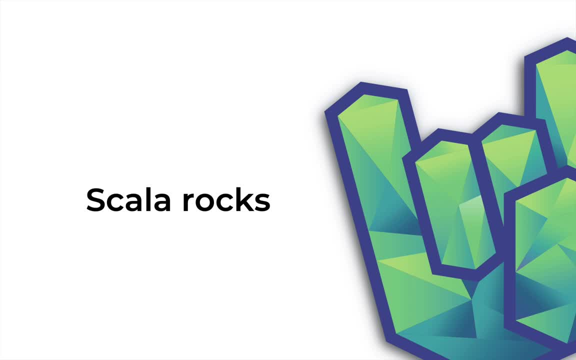 much more, but I noticed that the video was getting quite long, so I'm going to follow up with a second part to this video showing you the intricacies and the complexities of doobie in the next video. if you like this video, go ahead and click the like button for me and subscribe to the channel for more videos.